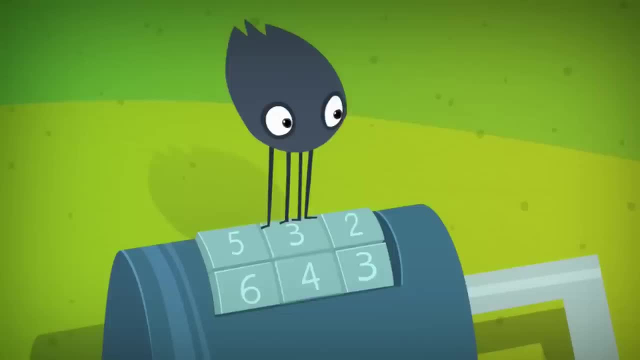 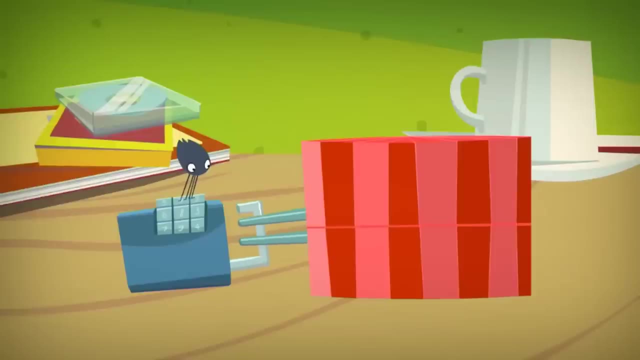 In the center of each disk is a hole with a notch When all of the disks are turned, so their notches line up in a straight row. the lock's pin can slide out freely. The pin can slide out freely. The pin can slide out freely. 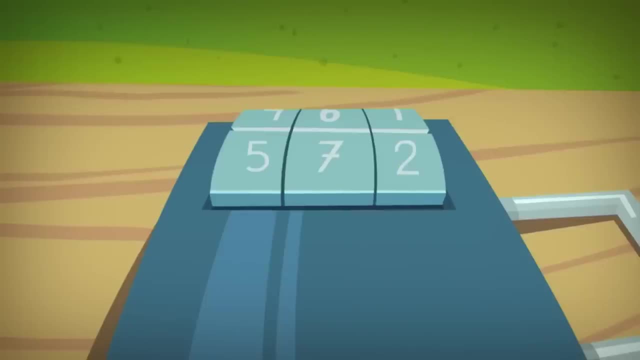 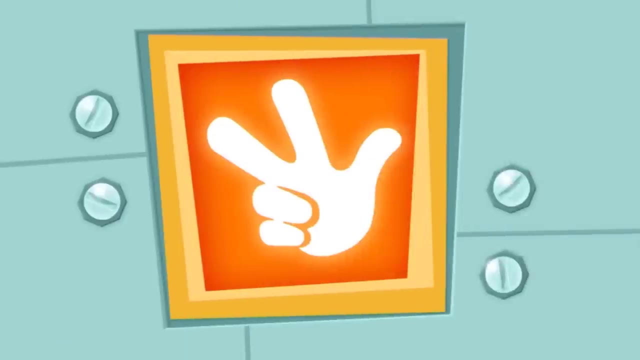 The pin can slide out freely, And to get the notches to line up, just turn the disks to the lock's code and the lock will open. It's that simple. Looks like we've got to take a look inside the lock, I see. 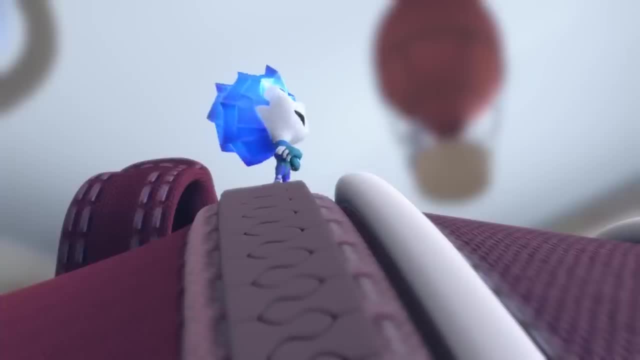 Nolik, where are you? There's work to do. I won't do it. I'm not going to help such a greedy boy. Nolik, won't you help me out here, And I won't be so greedy anymore. 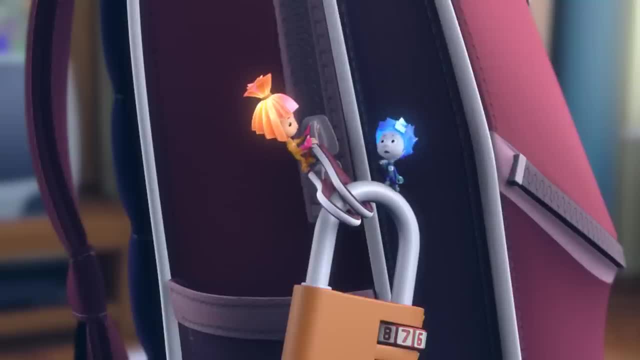 Alright, You broke me down. Omi, as soon as we're done, you're going to let me play with the game. Right, There's no room in here. Hang in there. We'll start turning the disks, one at a time, and you yell: stop when they're lined up. 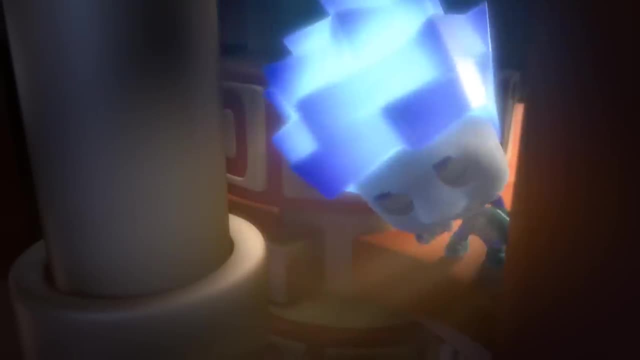 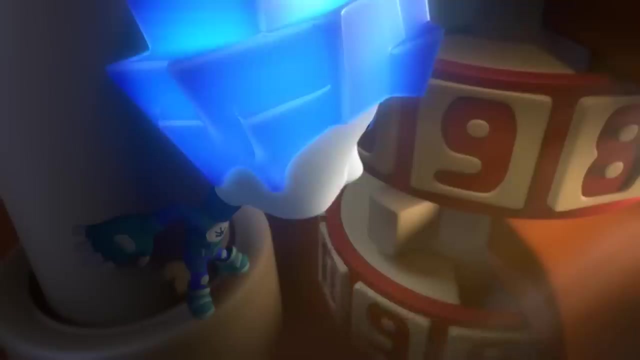 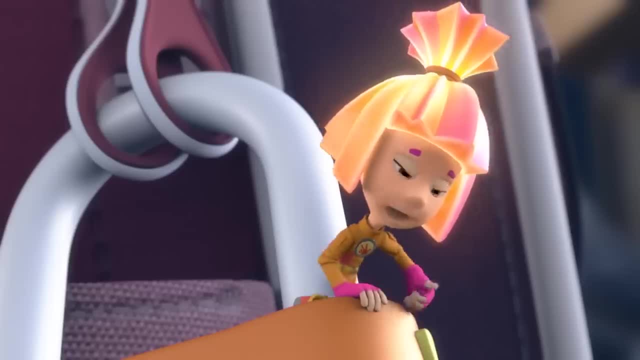 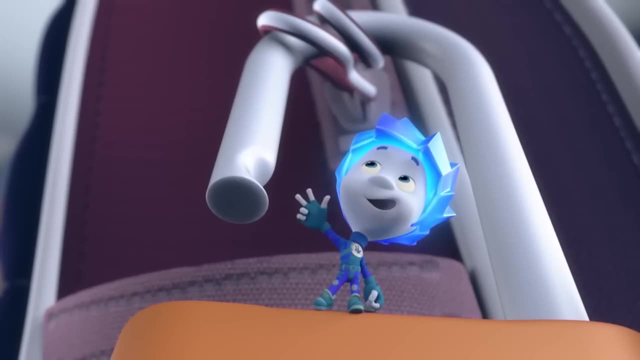 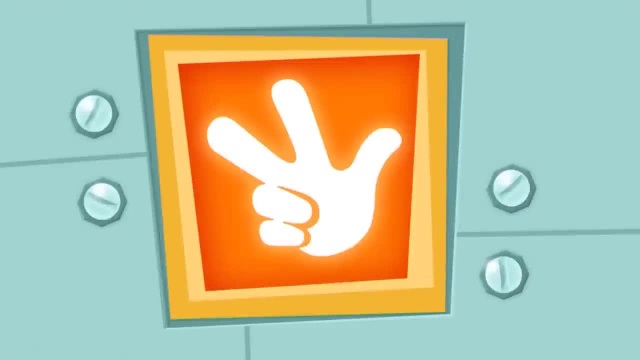 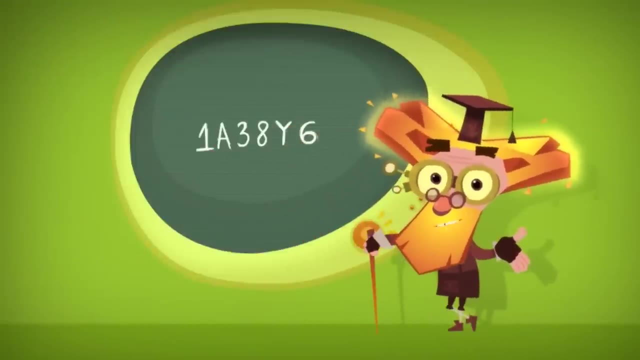 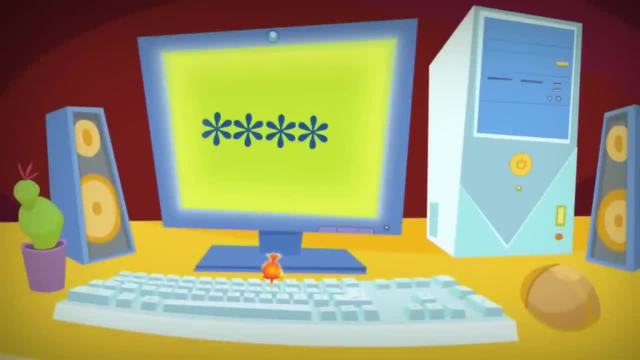 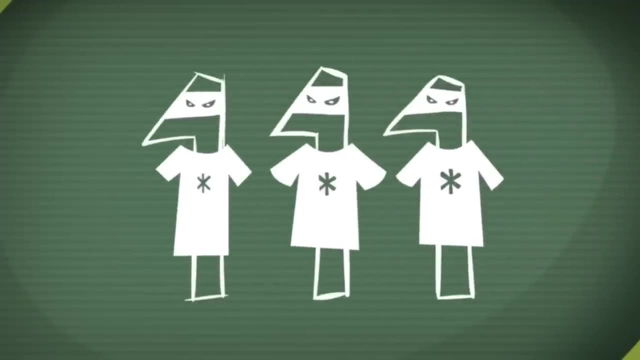 or the password. And to make sure your password's a really good one, here are some things you should know. Never choose a password that's really simple for someone else to guess, like one with numbers or letters that are all the same or are all in order. 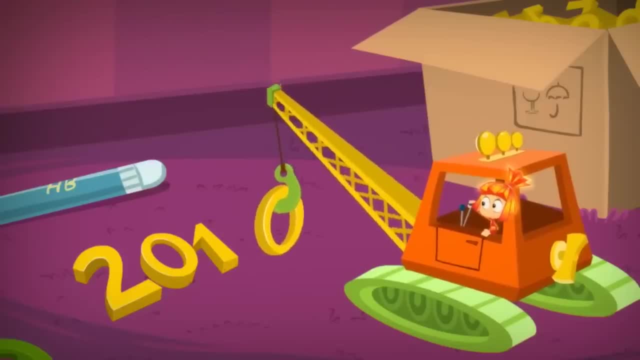 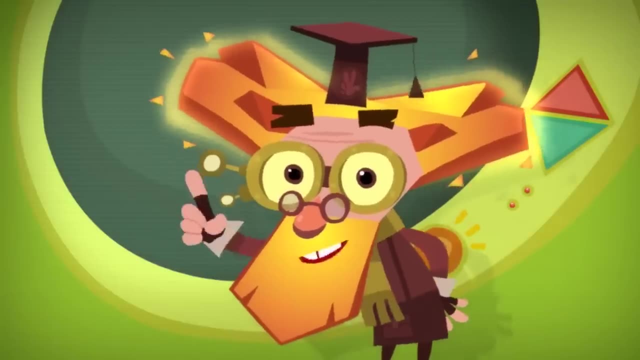 It's also a bad idea to make a password out of your birthdate or name. It's better to think of a password that's a bit more complicated, And don't forget your password once you come up with it. Write down your password on a piece of paper and keep it in a safe place. 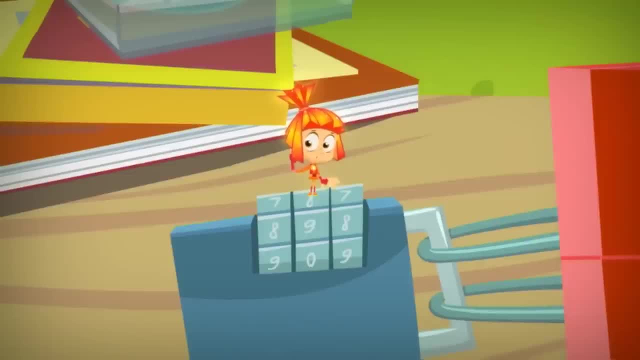 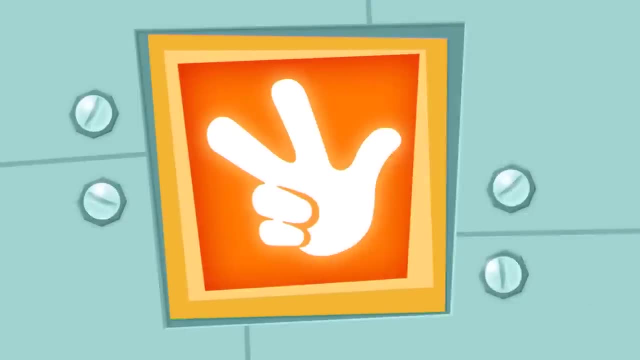 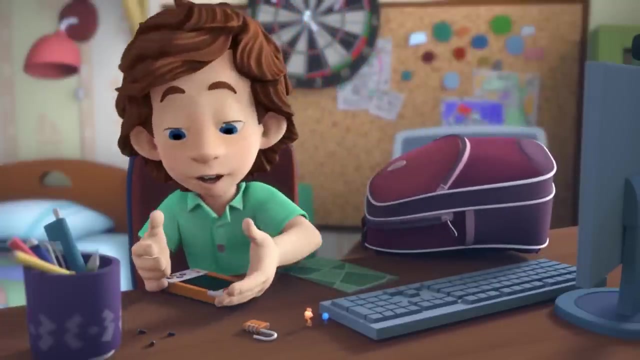 but don't show it to anybody else, And then, if you happen to forget your code or password, you'll be able to remember it with the help of that piece of paper. Bang, And why did you ever put a lock on your backpack? 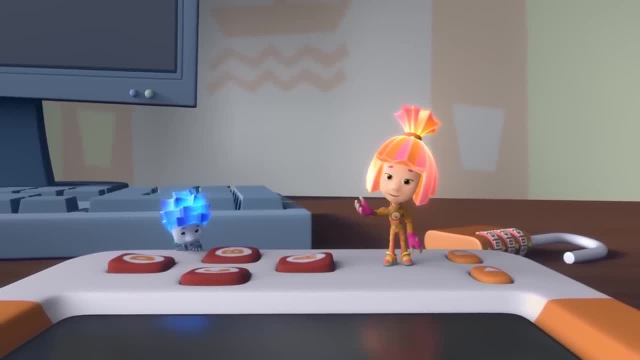 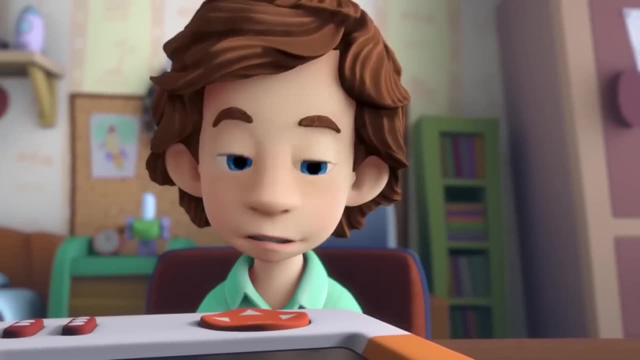 I was hiding the game from the other kids, Then why did you take it to school today? I wanted to show it off to my class And did you show it No way? If they would have seen it, they'd be like: 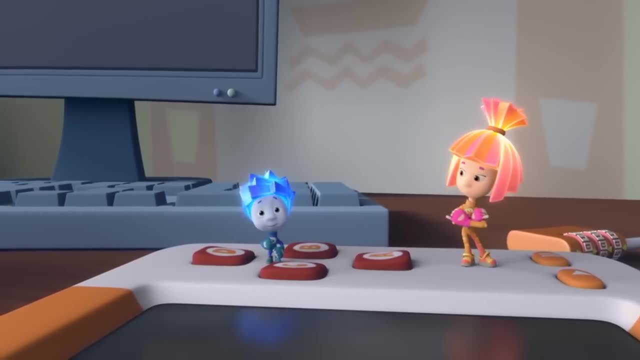 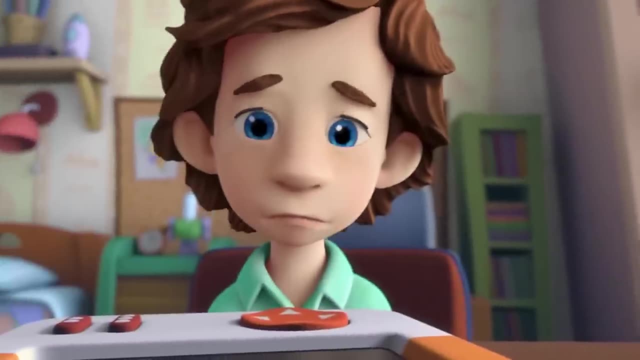 I want to use it, I want to play, And so you hid it and didn't show it to anybody, Not to anyone. Then why take it to school silly To show it off there? You're just some show-off. You're just some greedy…. 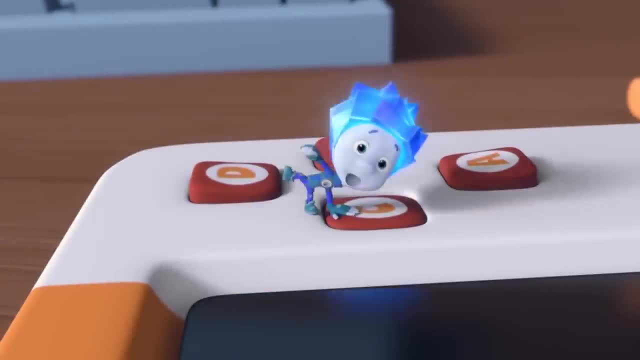 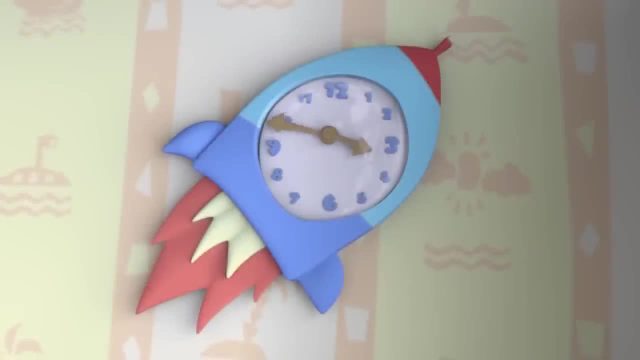 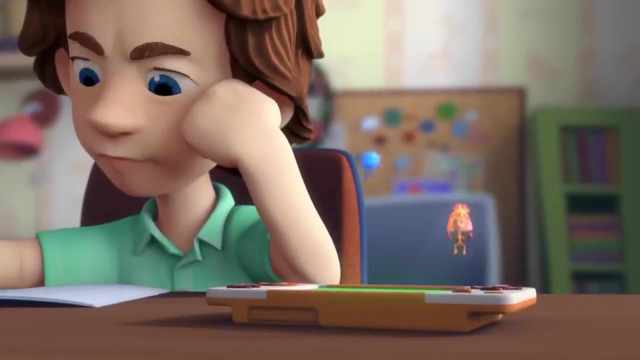 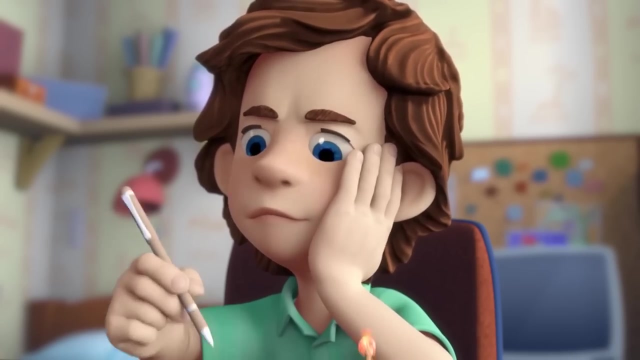 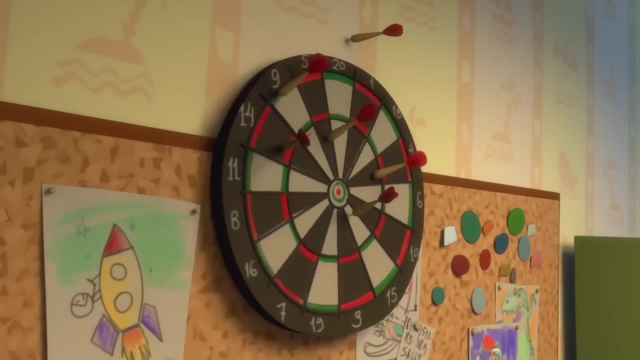 Oops, Sorry Once, greedy boy, Will you let us play now Play away. We're not bothering, you are we. Can you jump a little easier? You're shaking the whole desk. You'll miss for sure, No problem. Huh. 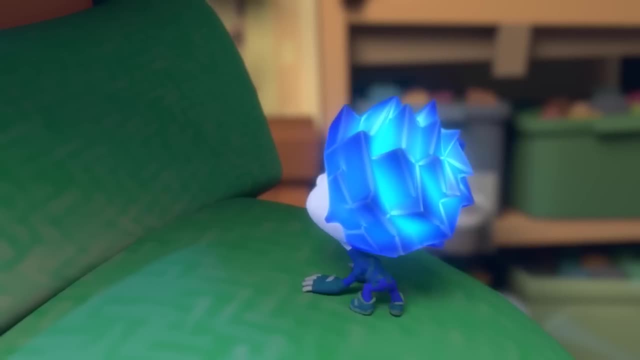 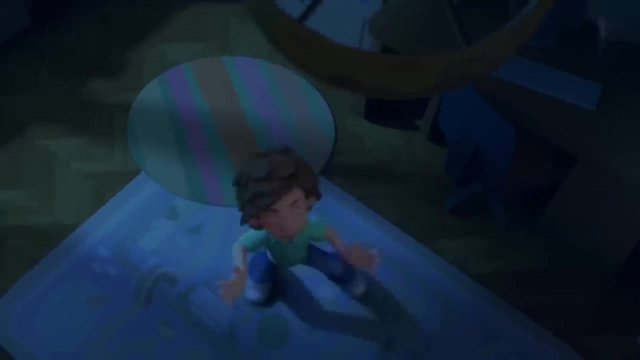 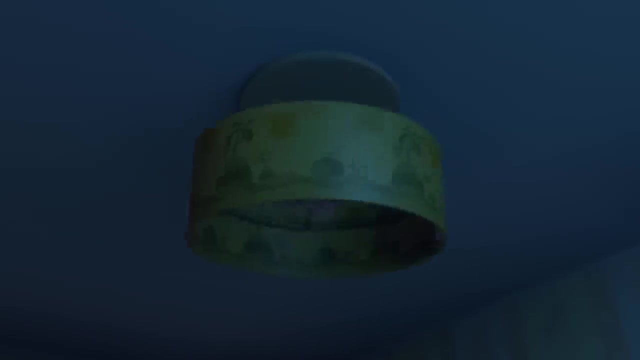 Anybody can do that, But I bet you can't do it if you tried bouncing the ball off the floor first. Just look, Oh, what are my parents gonna do to me? Maybe we should call Simka Simka. And what's Simka gonna do to us when she sees this? 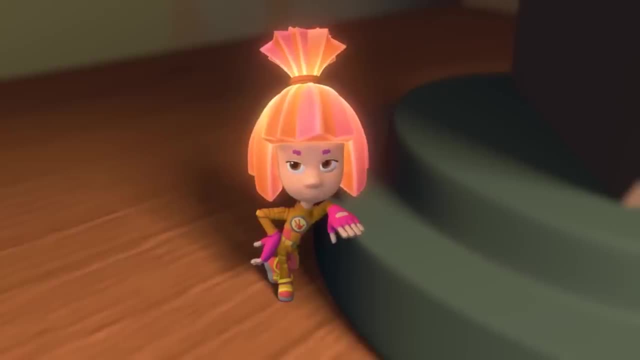 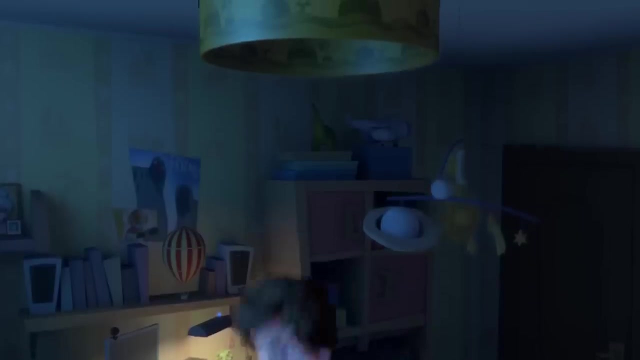 So got yourself in trouble. huh, You shouldn't be playing with a ball inside, And now we have your lamp to fix. But how? Only my dad can reach all the way up there. Why, just your dad? You have a hot air balloon over there. 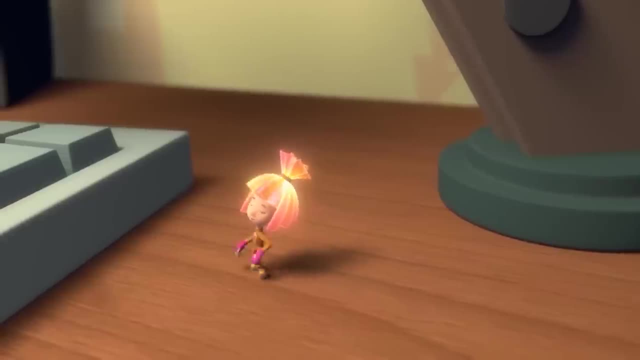 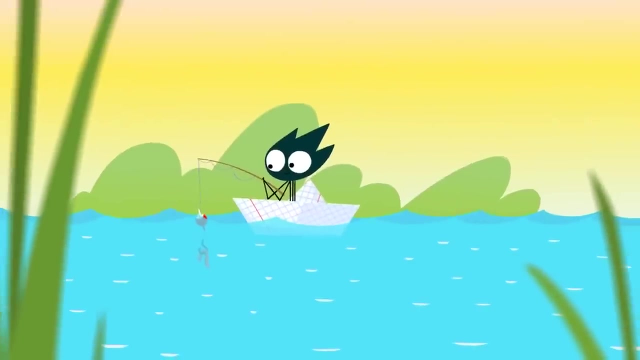 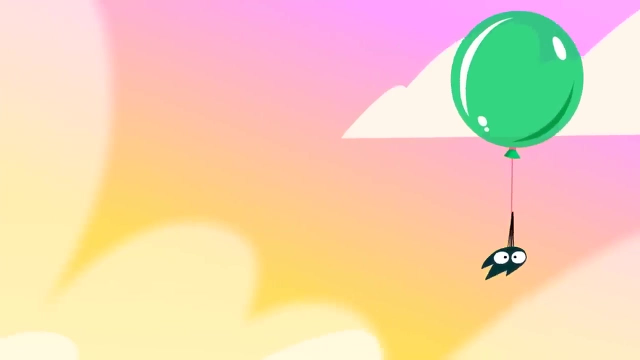 That doesn't fly, It's just a toy. see, Well, it might be just a toy to you, but for us Fixies, it's absolutely real. If an object is lighter than water, it floats up to the surface, And in the same way, if something is lighter than air, it floats upward. 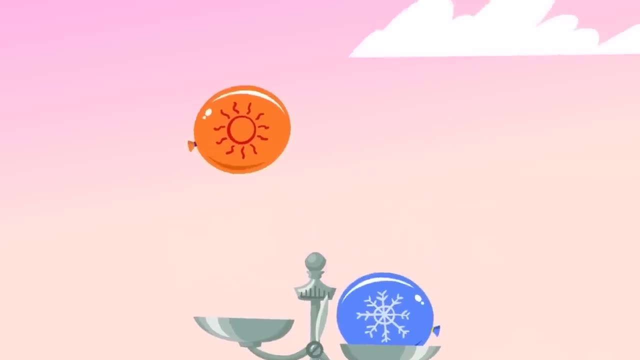 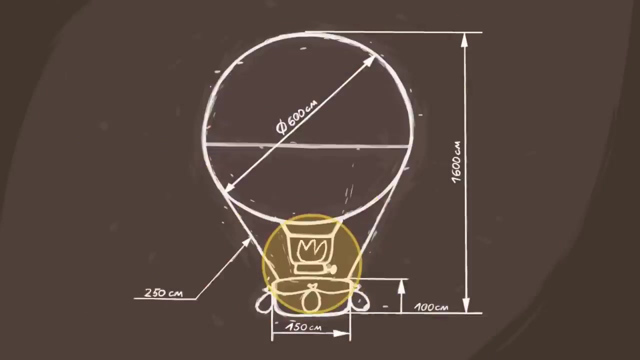 Did you know that hot air is lighter than cold air? Well, it is, And that means if you warm up the air in a balloon, it will float up. Hot air balloons use special gas burners to heat up the air inside of them. 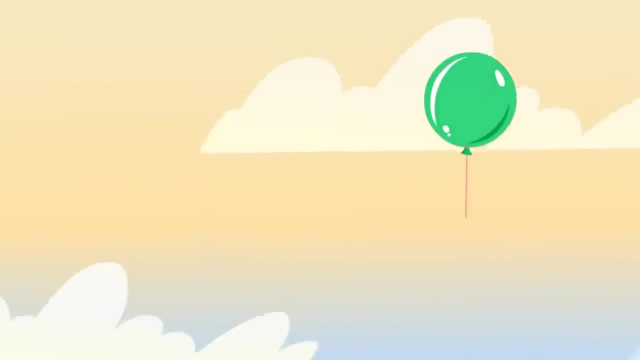 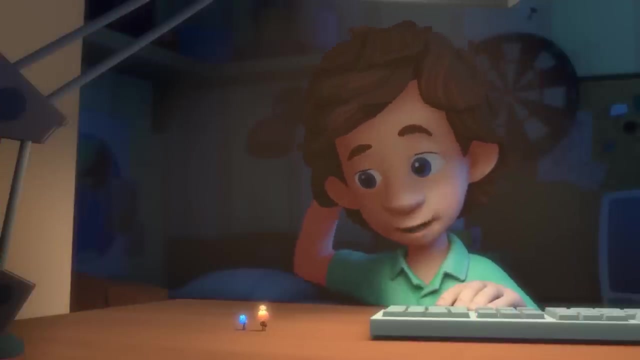 so they will get lighter, And the bigger the balloon, the more people it can take up into the air. I know what you're saying, but where do we get a burner? You think Fixies don't have their own burners? Ha, Sure, we've got them. 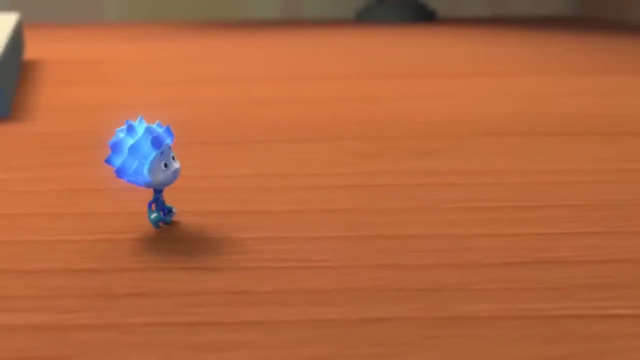 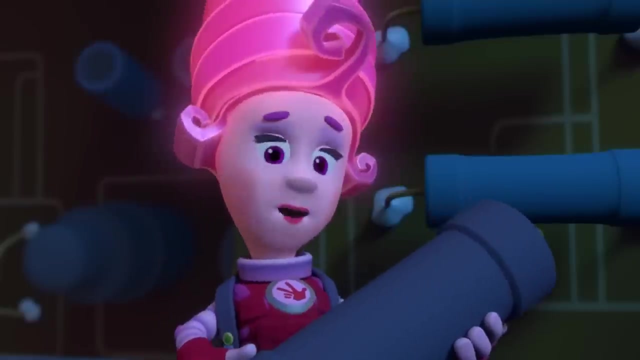 Bring it down here and I'll go talk to our parents. No, no and no. The human child must never see us. Listen now, Simka. We already don't approve of him seeing you and Nolik, He won't look. 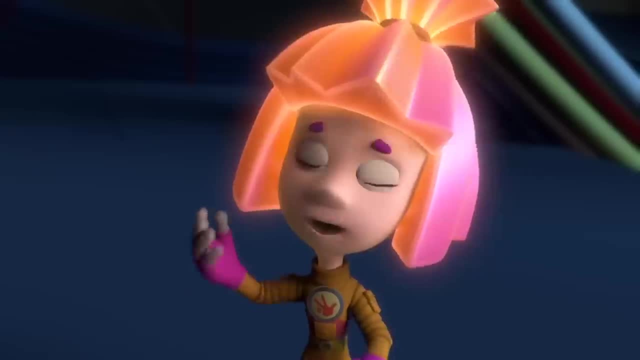 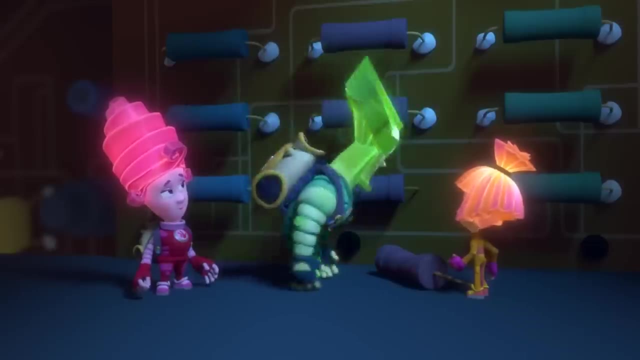 Pappas, please, You're the one who told us how you dreamed of flying, since you trained to go into space. Yeah, For two years I waited on standby, but I never went up. And you've never flown on a hot air balloon either, honey. 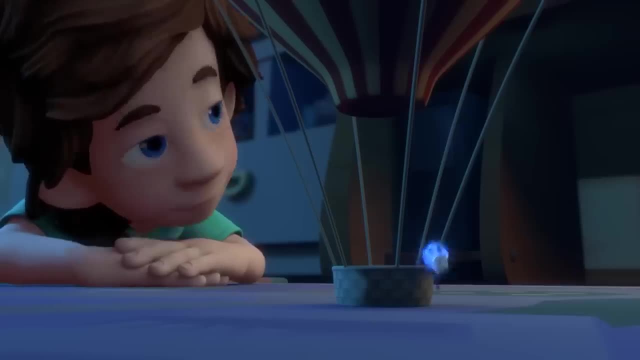 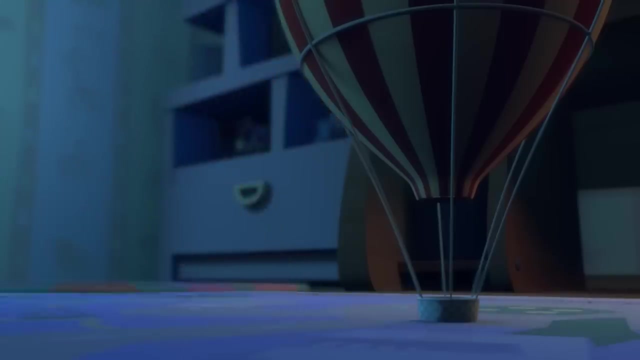 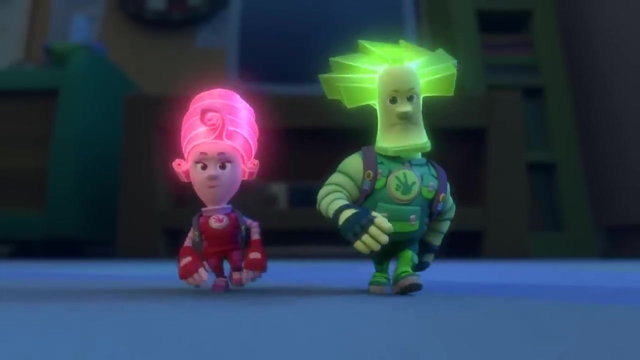 So let's call it a deal. I talked them into it. There's just one condition: You can't watch, OK, You can come in now. You can come in now. OK, Here I come. I'm ready, Here I come. 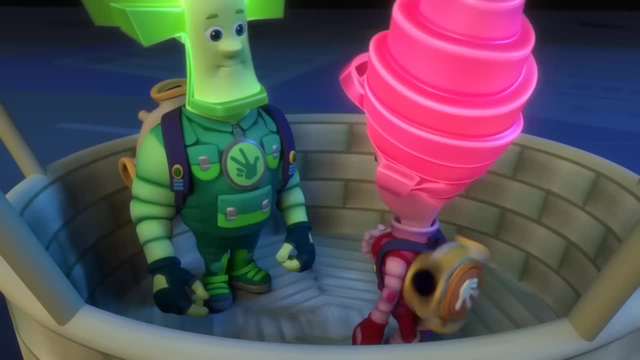 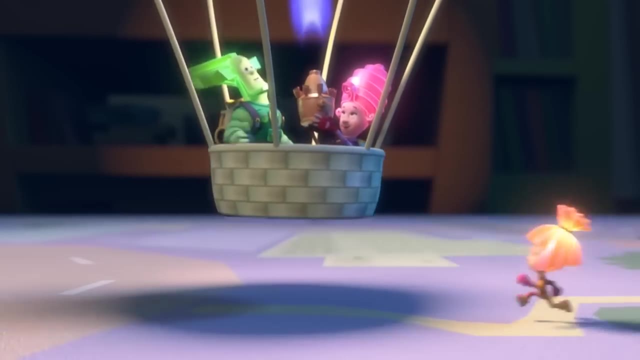 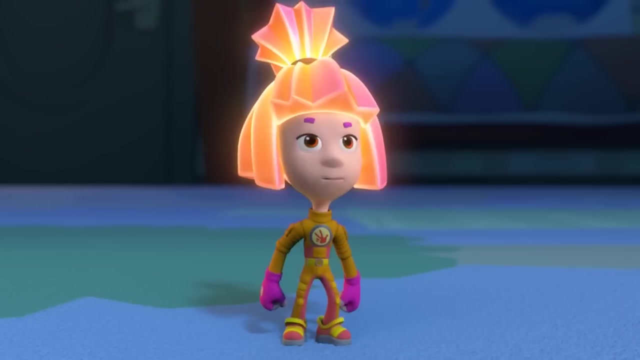 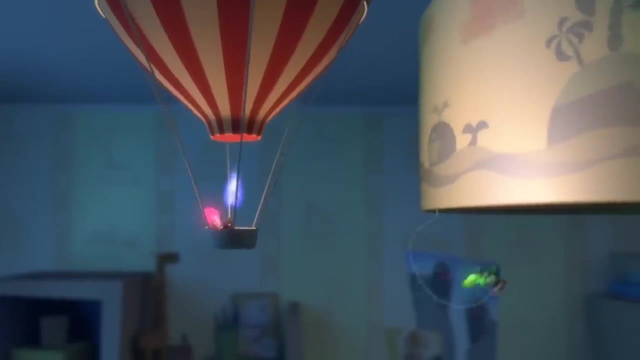 Now prepare the burner Coming right up, Permission for take-off. Permission is granted And off we go. Hooray It's flying, Don't you peek, Turn around. Oh, it was an accident. I'm going to evaluate the damage. 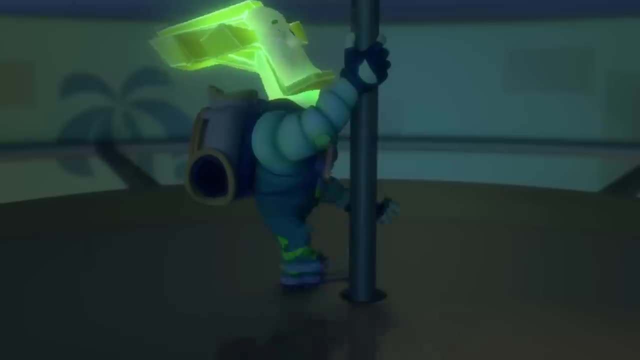 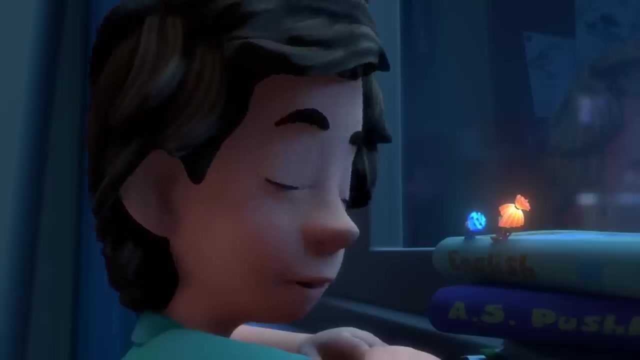 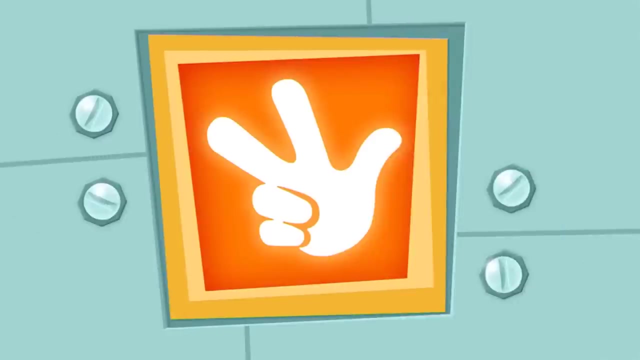 Maintaining proper altitude. So they've reached the spot. Air balloons are really awesome. I wonder who figured out how to do that. It was the Montgolfiers. The hot air balloon was invented in the 18th century by the Montgolfier brothers from France. 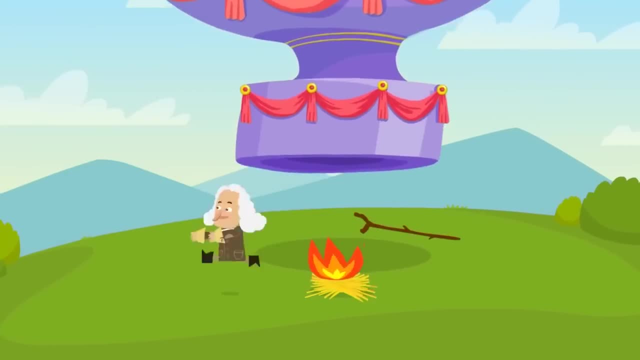 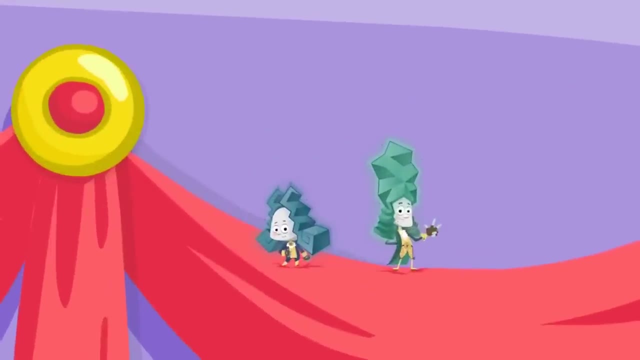 In those days there were no gas burners, so they heated the air inside the balloon by burning straw. At first there were no passengers on their balloon, Not counting the Fixies, of course. I mean how else could a balloon get up in the air without them? 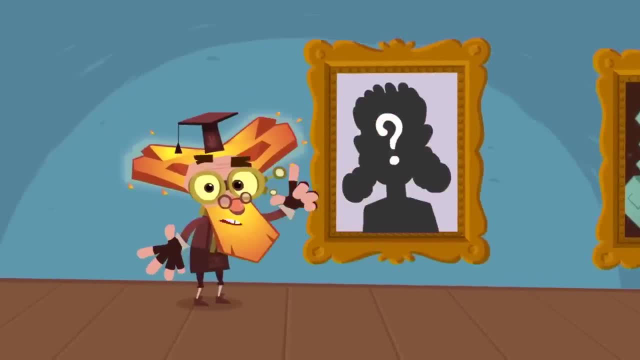 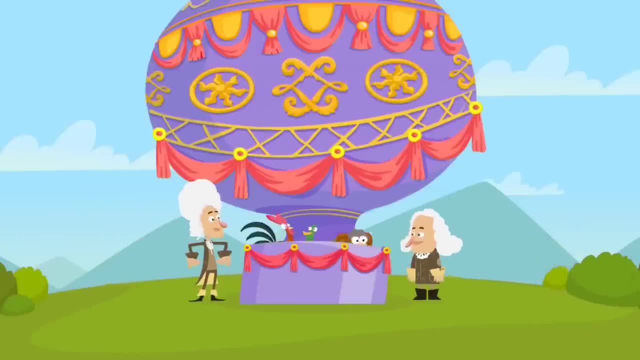 Unfortunately, the names of the first Fixies who took that flight were not recorded in the annals of history. Following the Fixies' flight, the next passengers were animals- A ram, a rooster and a duck- And it was not until those three safely landed. 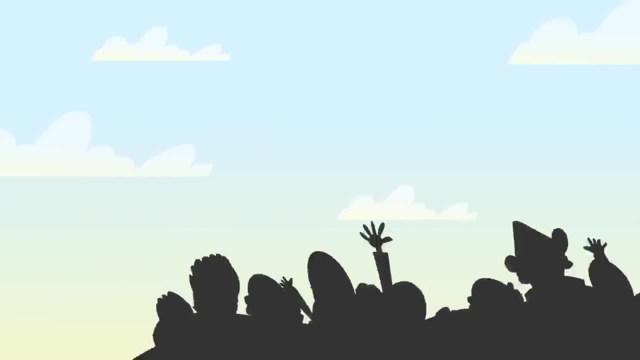 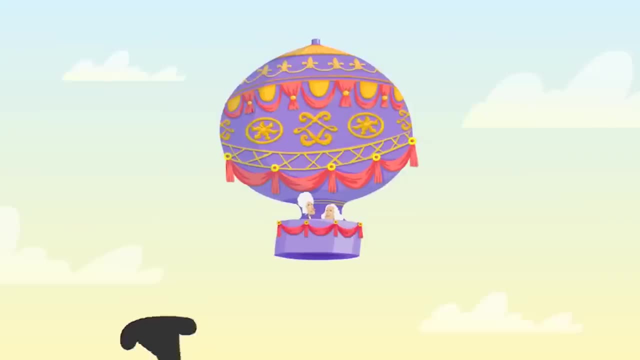 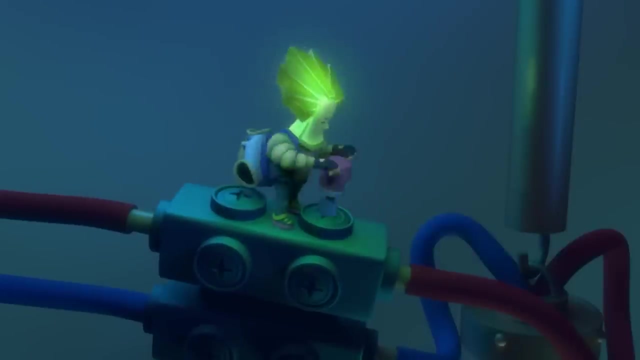 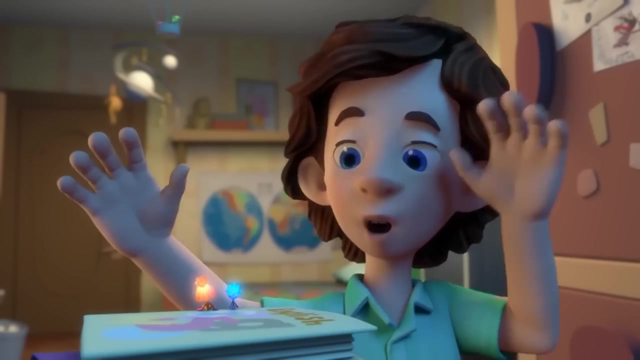 after flying a full four kilometers, that humans dared to fly in hot air balloons themselves. Ever since their invention, hot air balloons have also gone by another name: Montgolfiers, Hooray, Hooray, Tideesh, Tideesh. 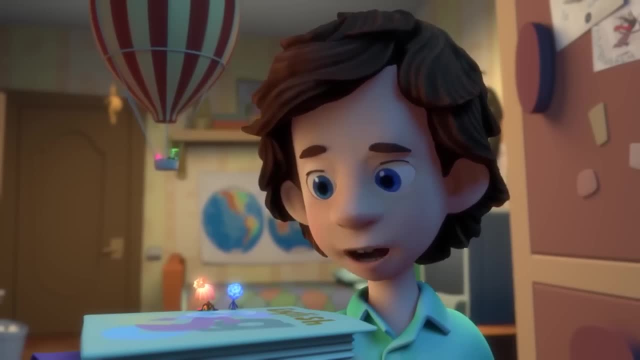 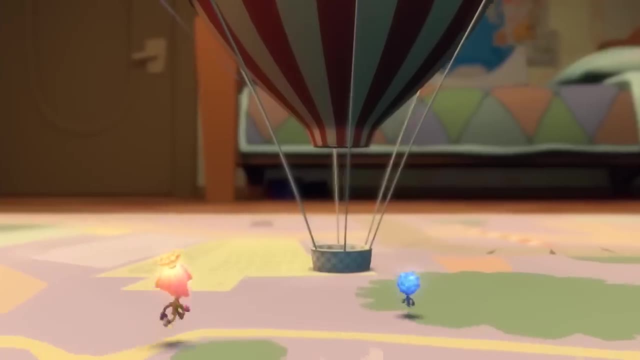 All right, Simka, please let your parents know that I'm so very thankful. Okay, By the way, now you can turn around. You know, Simka, let's fly the balloon, just like them. There's no way, Nolik. 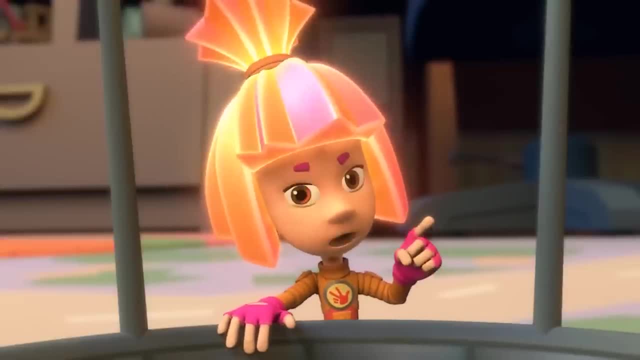 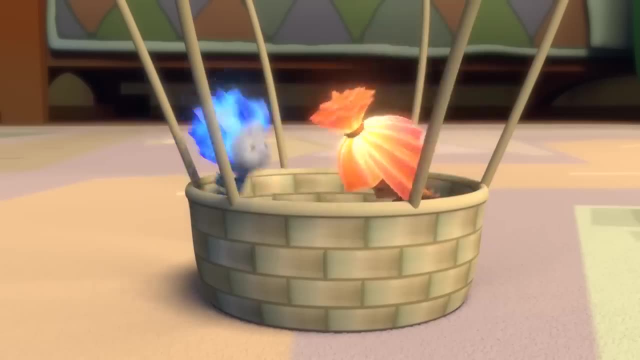 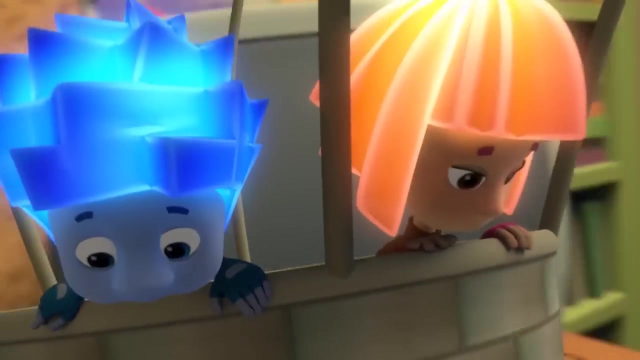 We would need to use the burner, and kids aren't allowed to play with fire. I'll give you a ride. Look, I still need to put it back up on the shelf, so climb up, Let's get going. esempio. 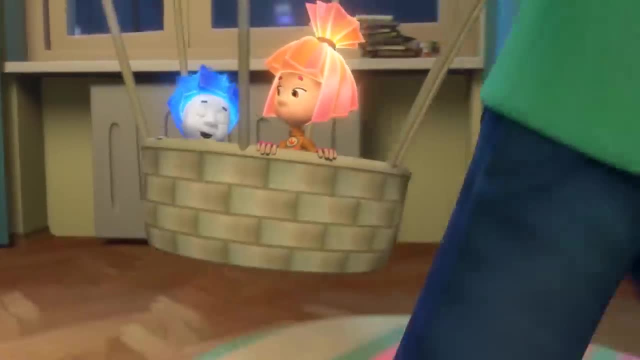 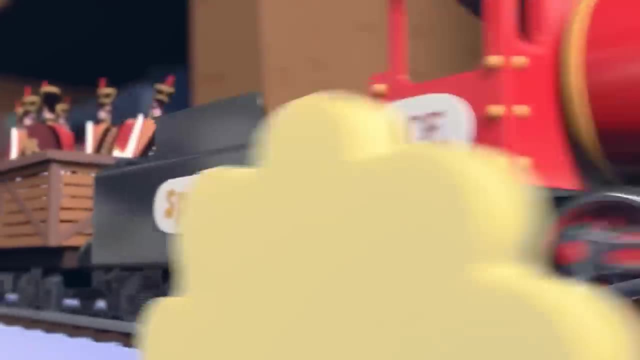 Tipo, Yo-ho, Hi-ya. No time in and let's do it. Hip-hip-hip, Ha-ha. Oh yeah, This is great, Simka. Look at us, We're flying, just like the Montgolfier Brothers. 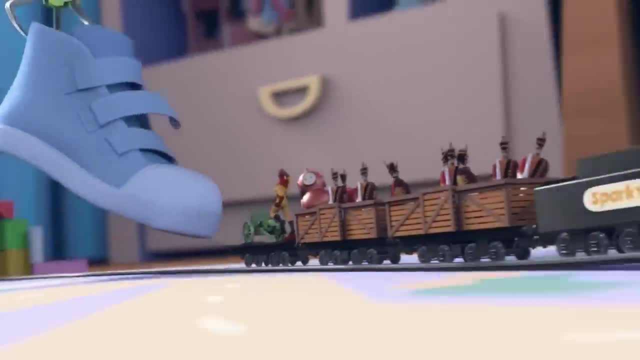 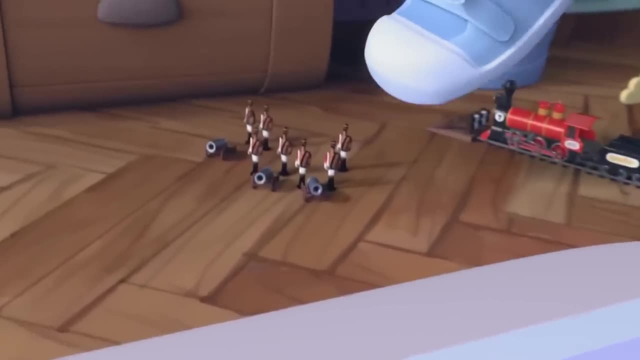 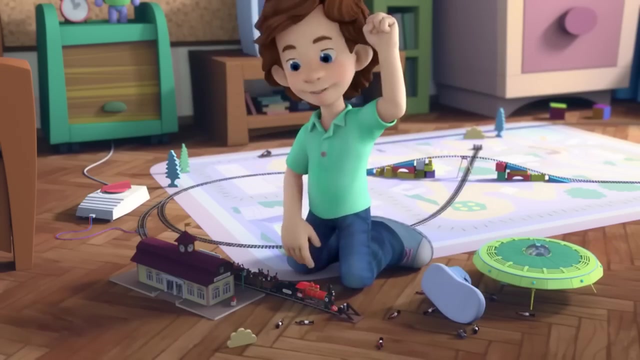 What do you mean? like brothers? Okay then, like brother and sister Montgolfiers. Suddenly, the Earth is attacked by an alien spaceship. If help arrives here on time, we'll be saved. Move faster, faster. Come on, get off the train, Move it, move it. 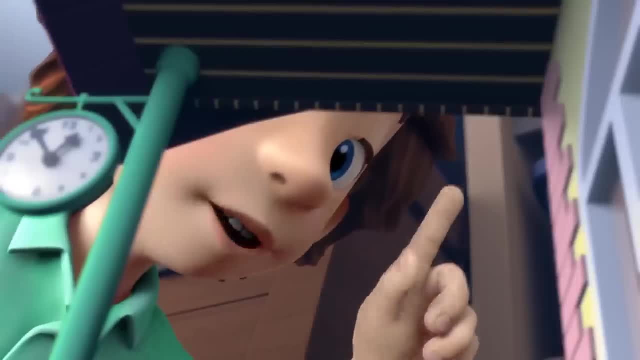 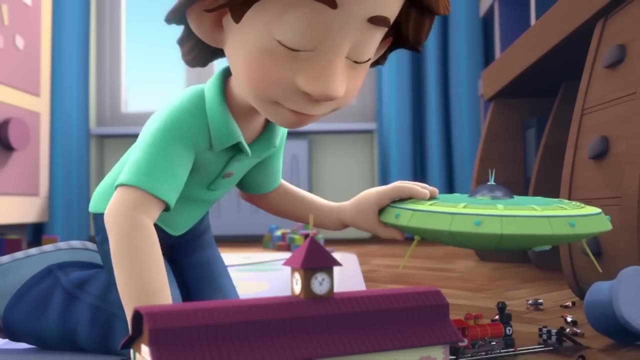 Tom Thomas, We came here to play. Ah, finally, you're here. I need some aliens for this game. What kind of aliens are you talking about? Just plain old aliens. You know the ones. They come, destroy the Earth and just about everything. 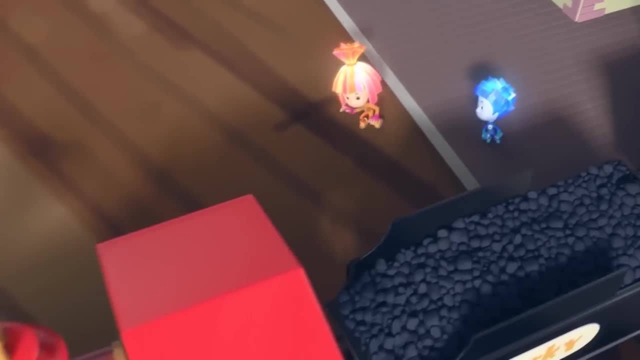 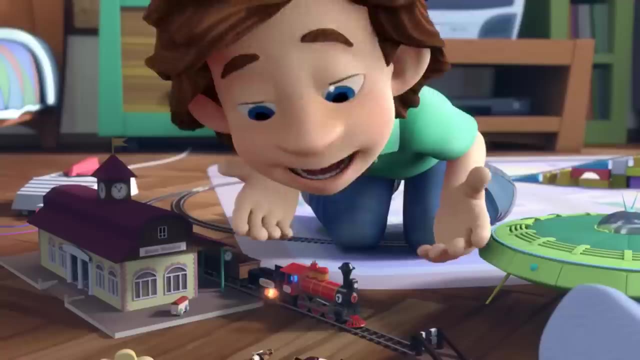 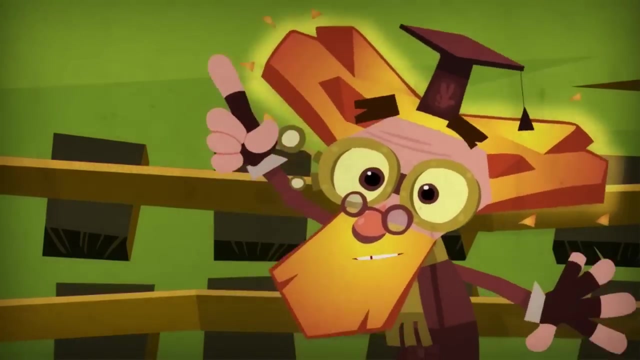 We don't want to destroy anything at all. Why can't we be the train engineers? Train engineers, You don't know anything about driving a train. Oh, we know plenty about trains. Humans invented the railroad long ago, but back then the rails were made out of wood. 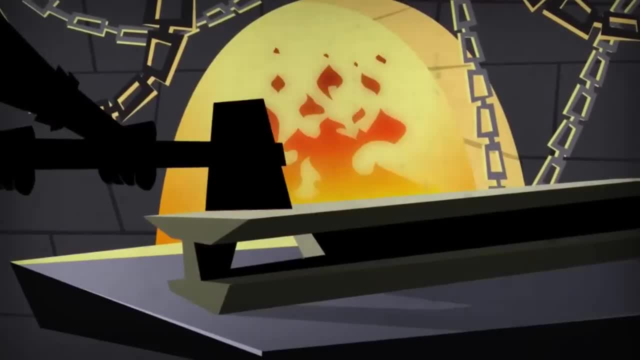 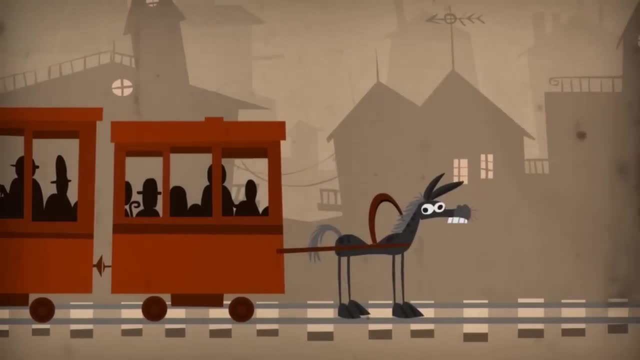 People didn't start making trains by using metal rails until the end of the 18th century, But the first railroad cars had no engines to give them their power. Instead, they used horses to pull them along. Later, horses were replaced by the steam engine. 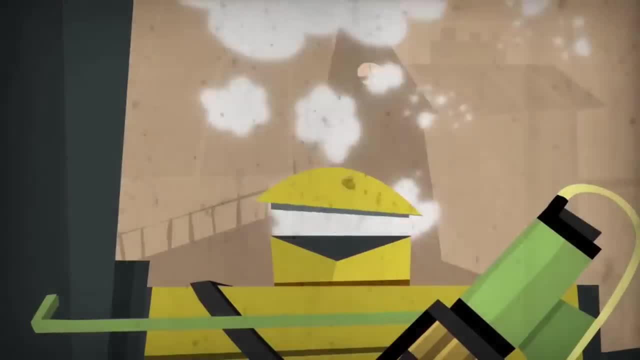 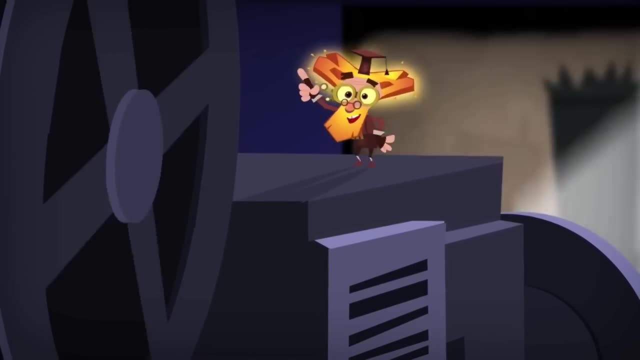 Wood and coal would burn in their furnaces to boil the water in the boilers, making the steam that turned their wheels. And the Fixies were there to help those trains go, making sure all of the parts could work together smoothly. Subtitles by Subtitle Workshop. 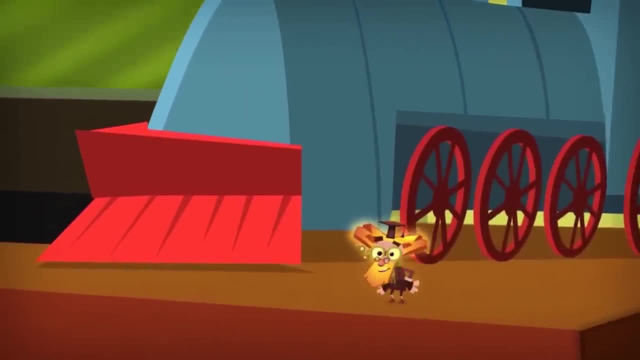 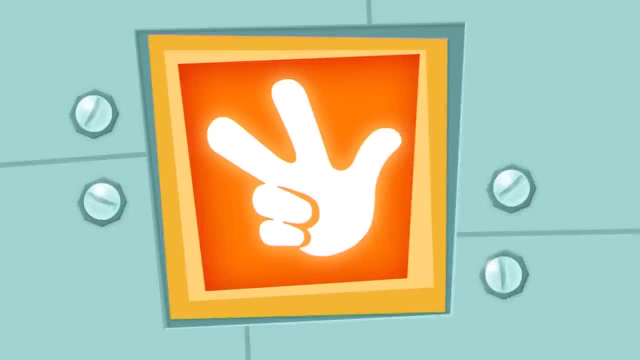 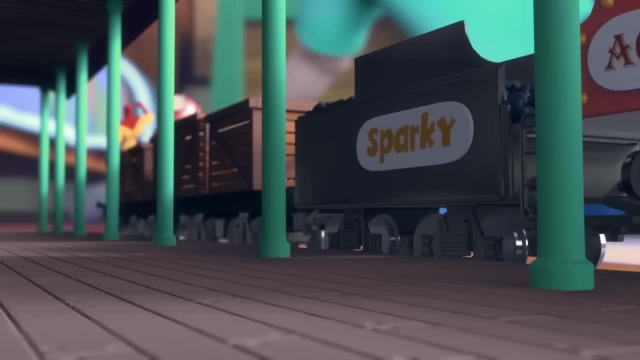 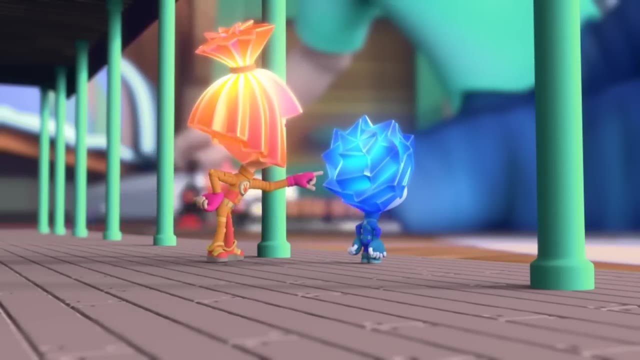 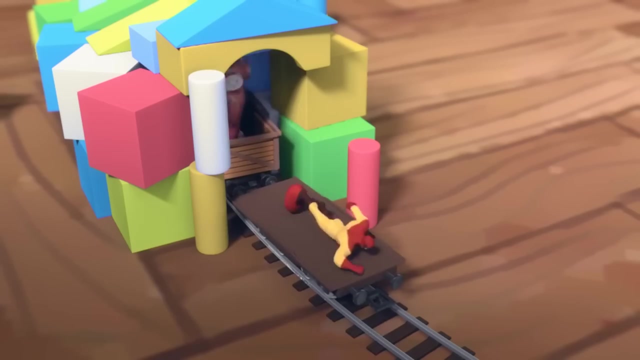 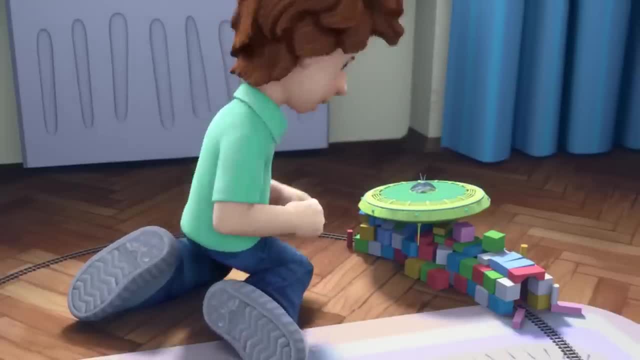 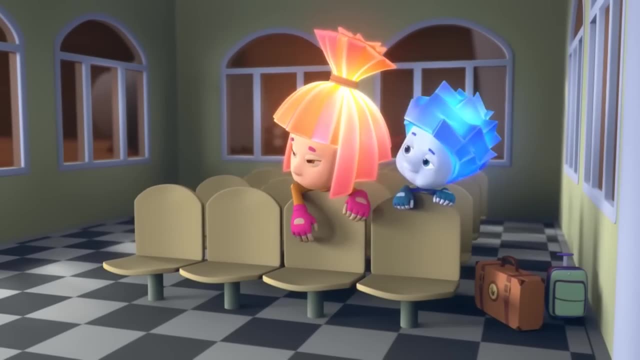 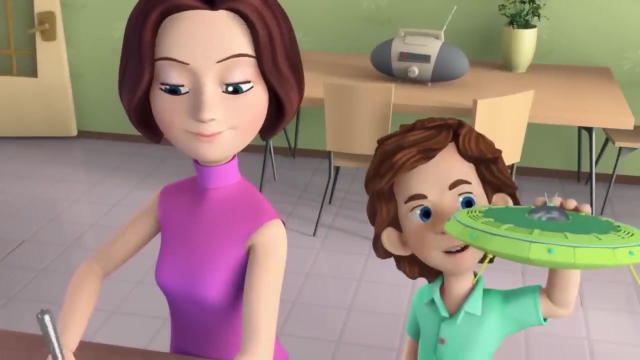 This doesn't help either. It's not going at all. Simka Nolik, Where are you? Did I hurt your feelings or something? Mom, is dad gonna be home soon? No, is something the matter? We've been attacked by evil aliens. 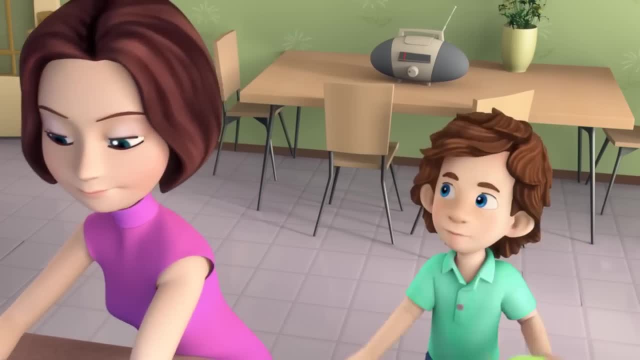 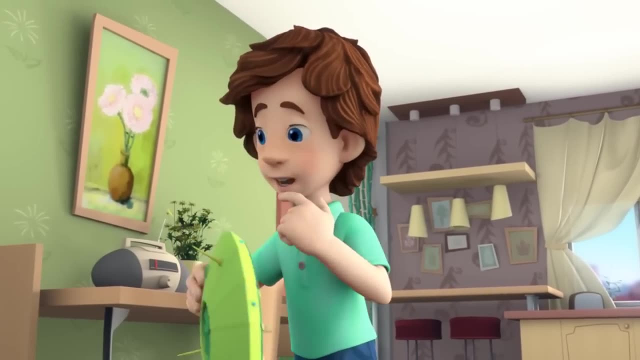 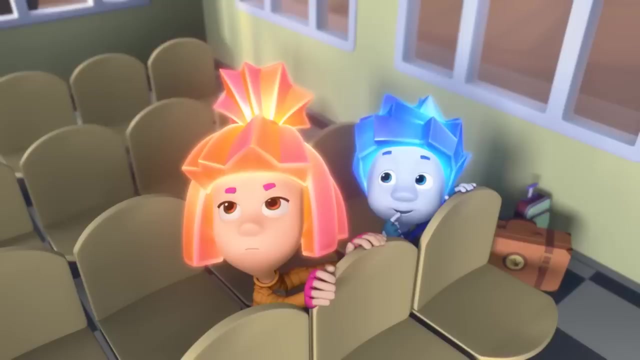 The train has to be fixed right away or we'll never escape them. You want some tea? I've got to think of something. Simka Nolik, I know you're in there. Please forgive me if I hurt your feelings. 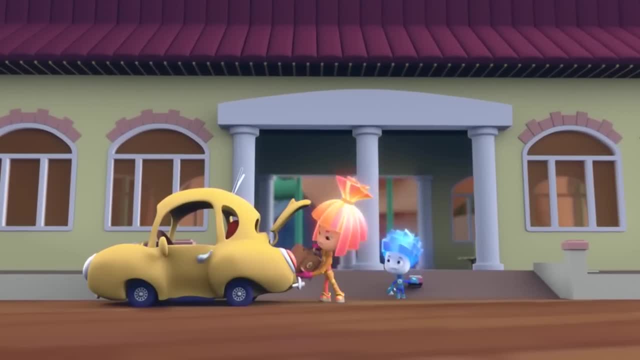 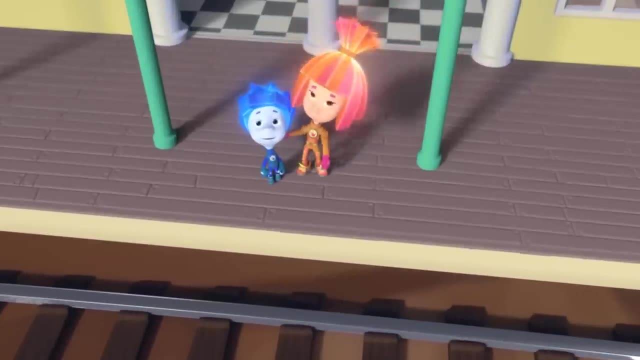 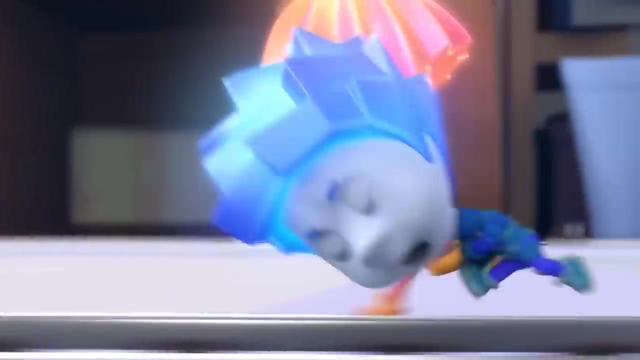 I'm really sorry. There's nobody but you that can save the world from the evil aliens. Alright, it talked us back into it. Well, let's go and check the rails. Nolik, follow me, I'm faster, Whoa. 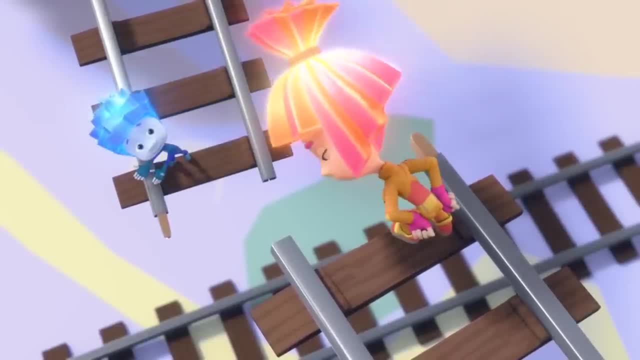 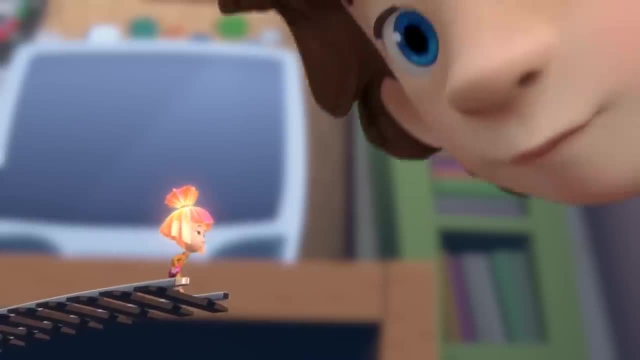 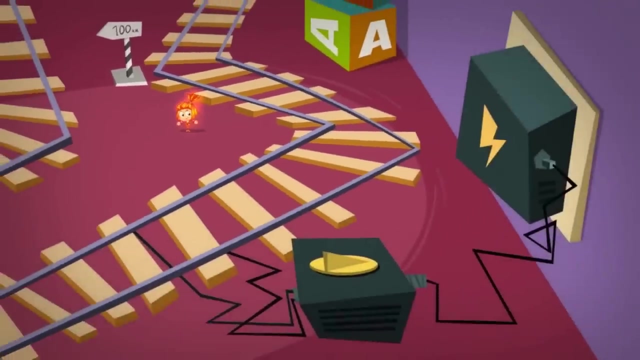 Well, so much for being faster. It looks like I found the brake. Tom, Tom, Thomas. The rails are broken, I know, and so You know, but that's why your train's not running Just like a real train model. trains run on electricity. 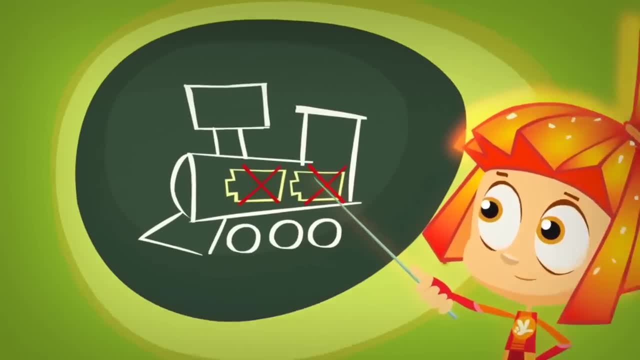 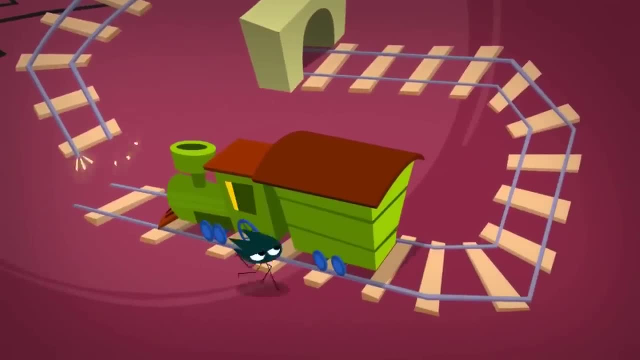 But there aren't any batteries inside the locomotive to pull the other cars. The engine gets its electricity from the rails. Each piece of the rail has a wire in it. If the rails come apart, the electricity can't flow through the track and get to the train. 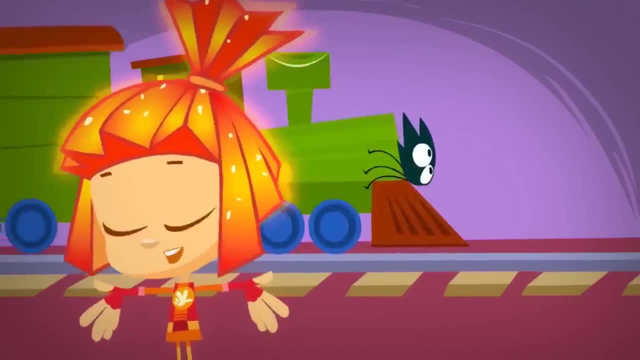 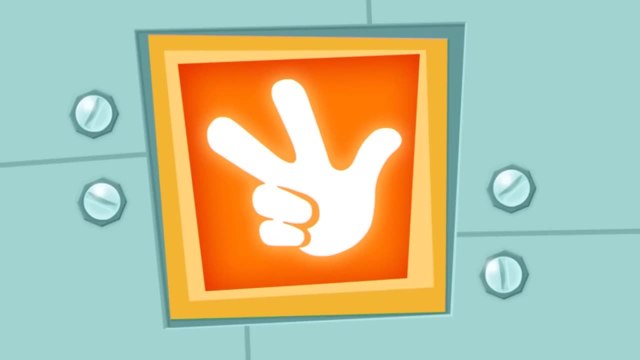 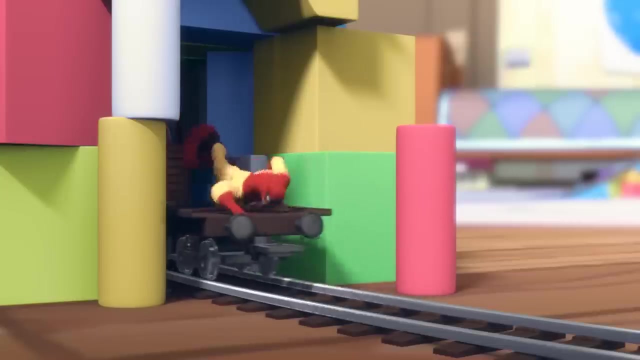 And without electricity the train's engine just stops going. So reconnect the rails and your train will run again. Uh-huh, Put them together. Ah, Yes, Hooray, The train's running Way to go, So will you play with me now? 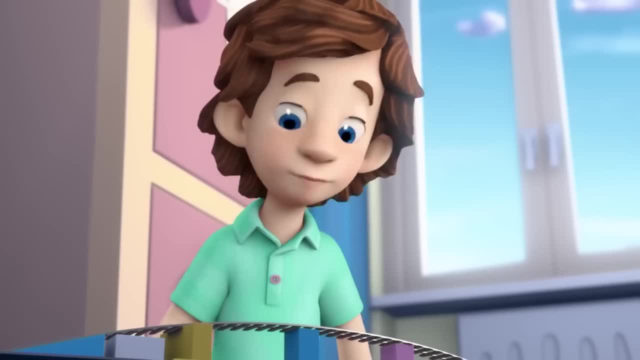 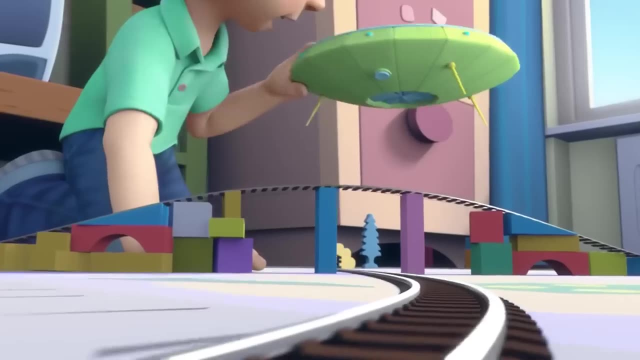 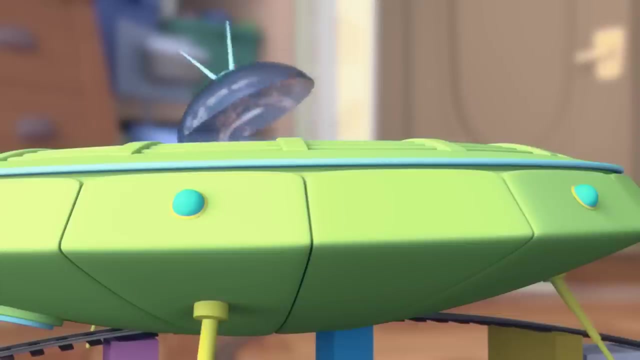 And which way are we playing this time? Whatever you want, I'm with you. The train's running. The train rushes down the track with no like as its engineer, when suddenly, from out of the sky comes an alien spaceship. Greetings to you, oh people of planet Earth. 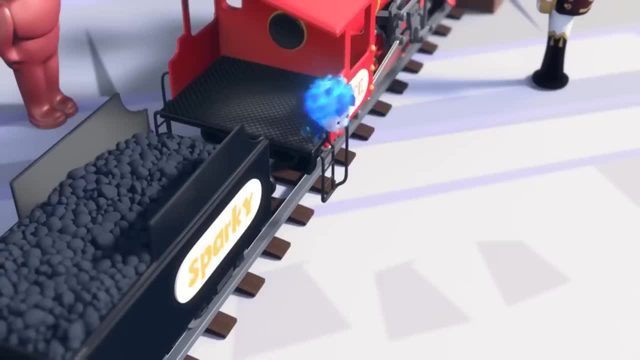 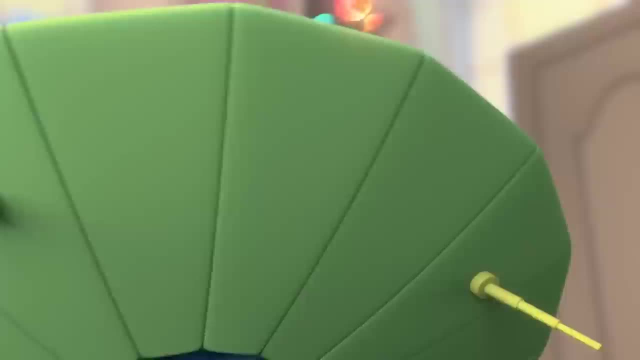 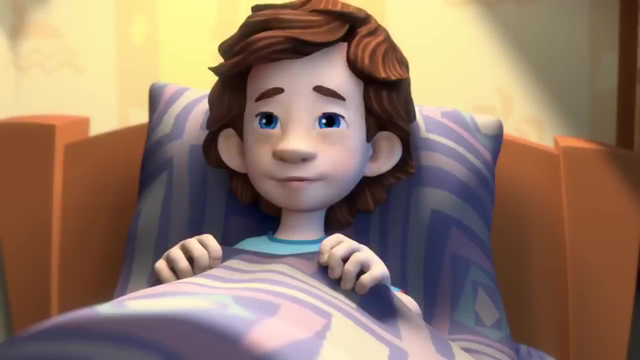 I come from far away, from another galaxy. Have you come to destroy everything? No, I've come to fix it all. Oh Yes, honey, only a thousand times or so. A Robotozoid R300 would just be the greatest. 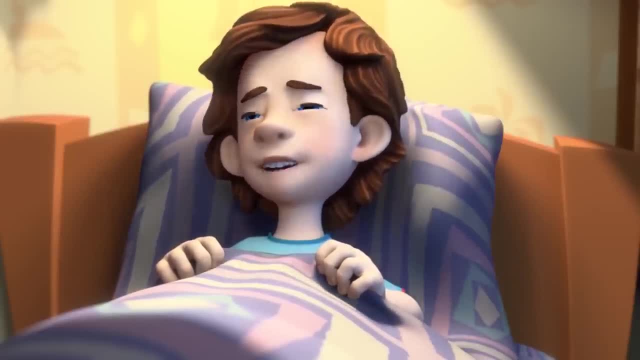 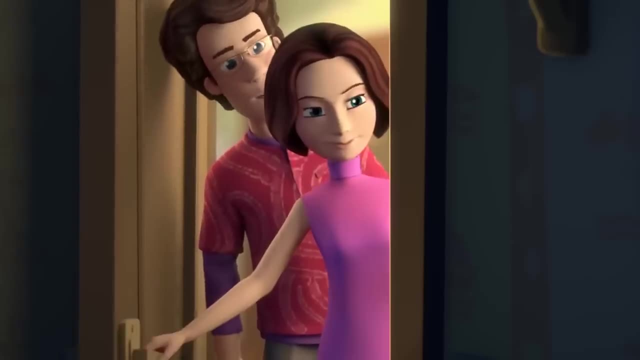 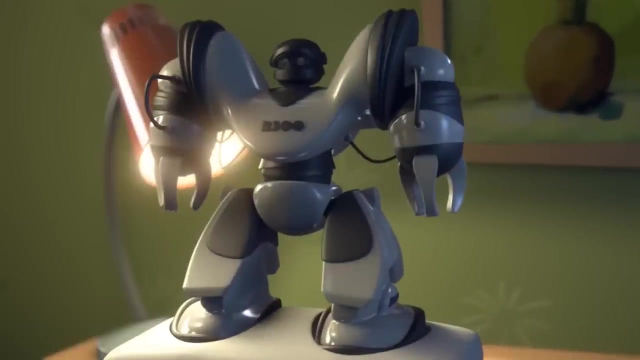 With MegaVision. I want it, I really do. Ah, I do. Well, tomorrow you'll find out, But now it's time to sleep. Tom Thomas, Wow, that is one great present. And we got Tom Thomas absolutely zero for his birthday. 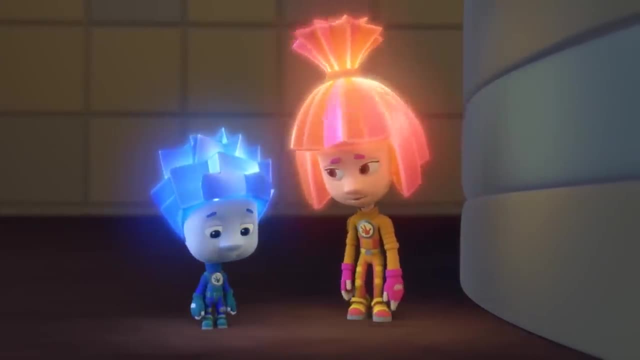 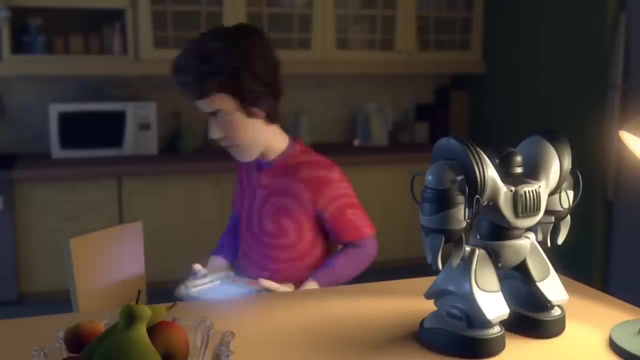 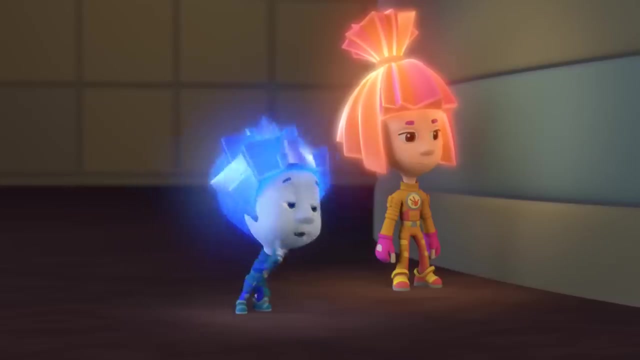 Ah, we're just terrible friends. I'm sorry, We're just terrible friends. So how does this robot work? OK, so let's give this a try, shall we? First we'll take a walk, And how does he have any idea where the robot's going? 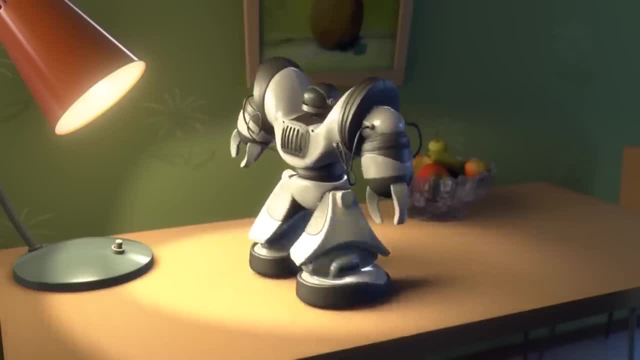 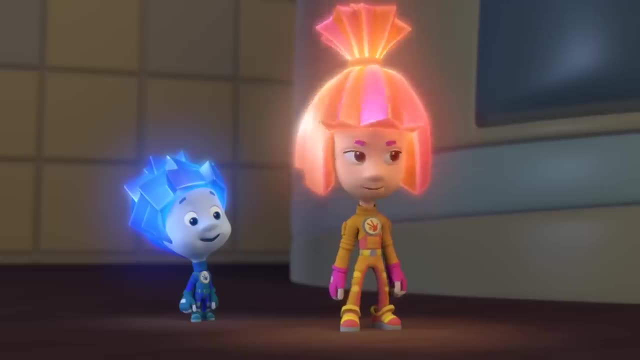 I can tell you, One of the robot's eyes is a video camera. The robot sends the picture to the screen on the controller so the player can see where the robot is going. Yeah, And that's just one thing. they know how to do. 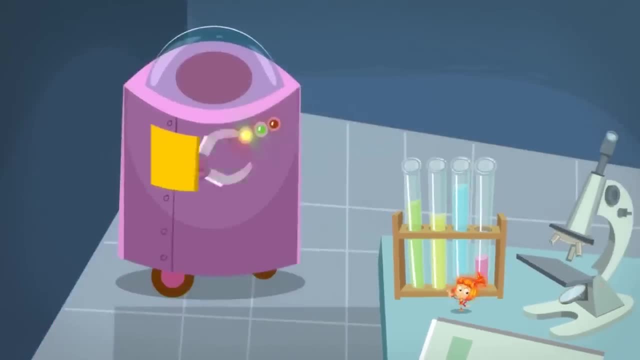 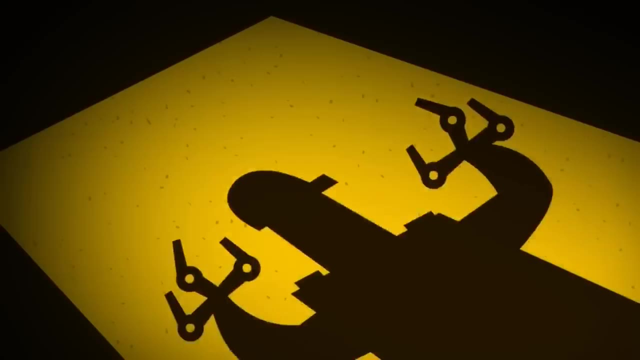 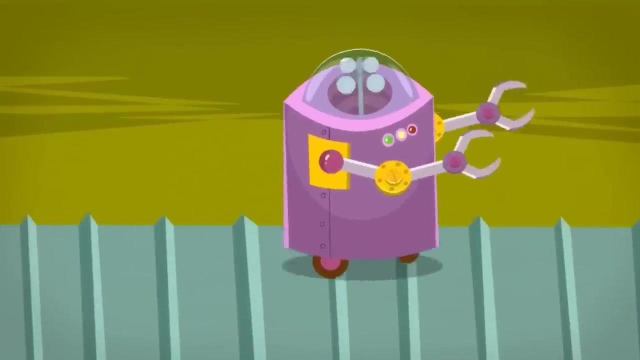 Yeah, A robot is a smart machine that can do very difficult or dangerous work for humans. With its strong metal arms, a robot can move heavy objects or put together carts to build cars and other machines. Robots are often sent into outer space or to the bottom of the ocean to help scientists. 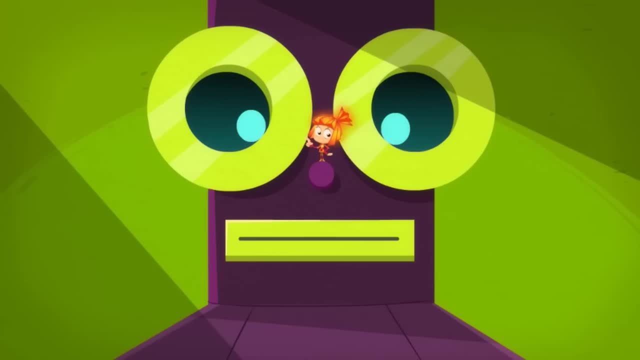 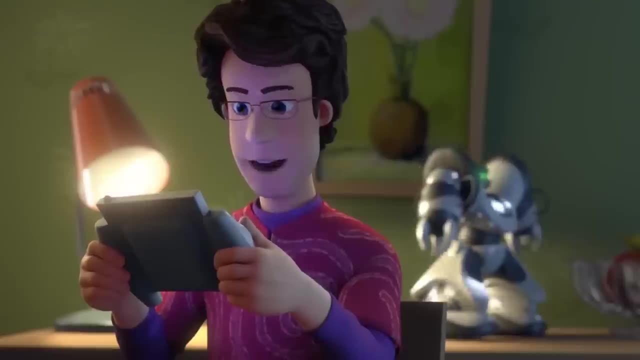 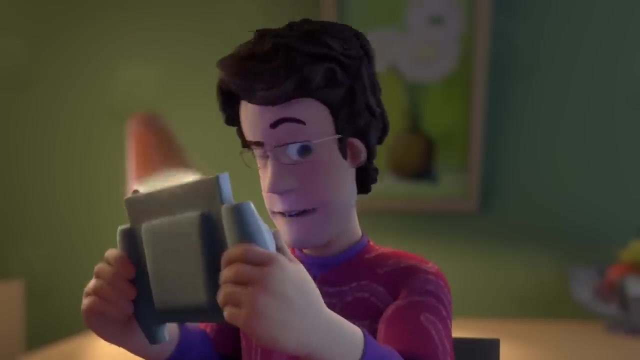 There are also robots that can understand what people are saying, And robots that can talk and even make jokes, Just like people. I've got it. Now let's turn you around. Ah, What was that? Uh, look, You know. 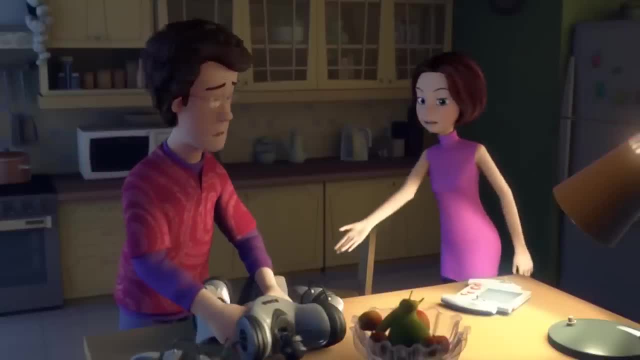 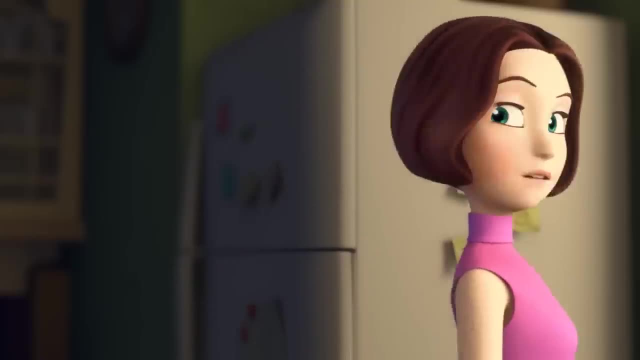 He destroyed him. Nolik, stop, You were playing with that, right? You think Tom will notice. Oh, I know what you're doing all night. I'm off to bed. I'll get him to work. I'll stay up until I do. 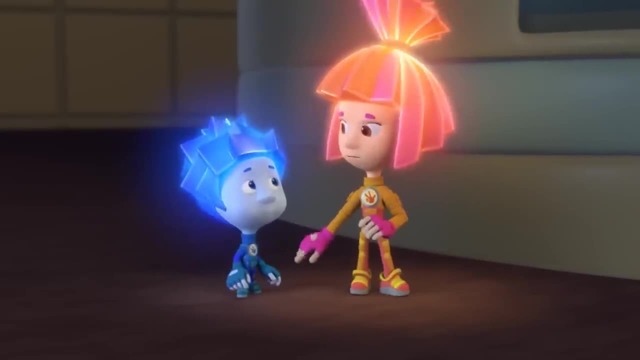 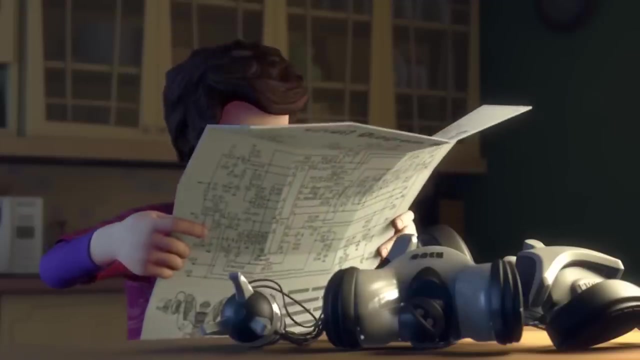 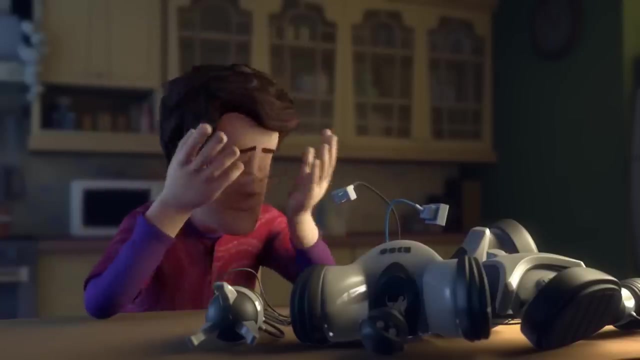 See you, Simka, let's try and No, we're going to need some help When your TV has broken, When your cell phone has croaked, Your laptop's barely working, The kettle's had a stroke. Don't ask us where we're going. 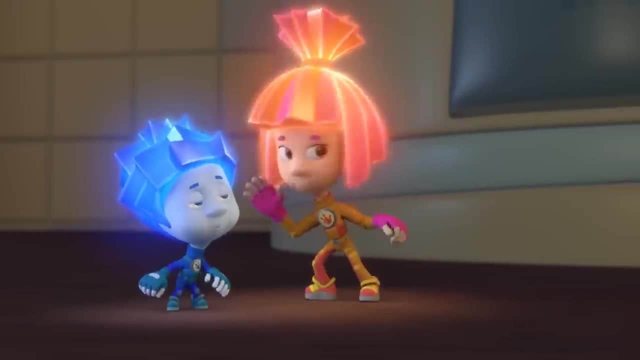 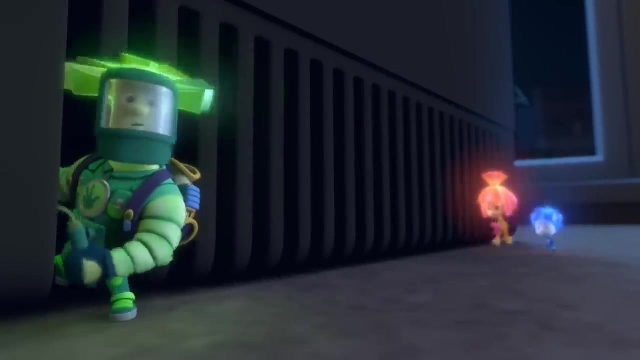 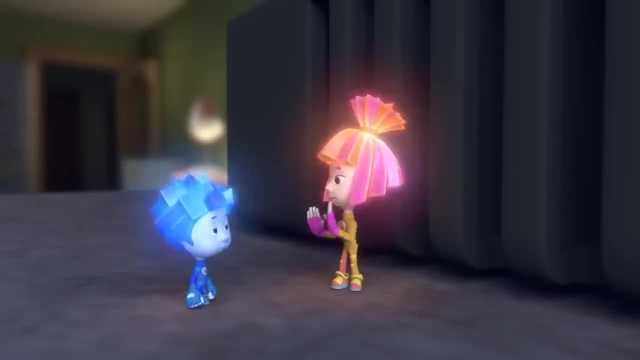 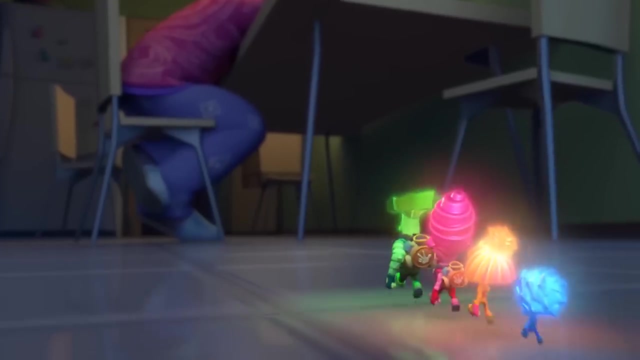 Inside we'll be Tideesh To fix what's wrong. Tideesh Till it runs strong In gadgets and devices. Our work will never end. Appliances are fickle. They need a loyal friend At morning, noon and midnight. 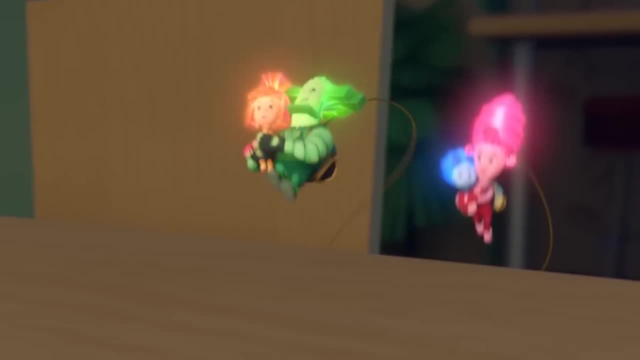 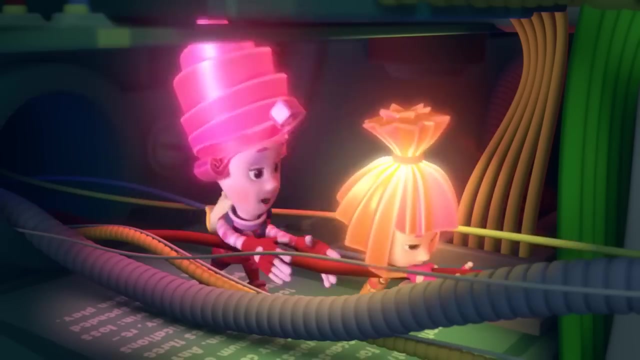 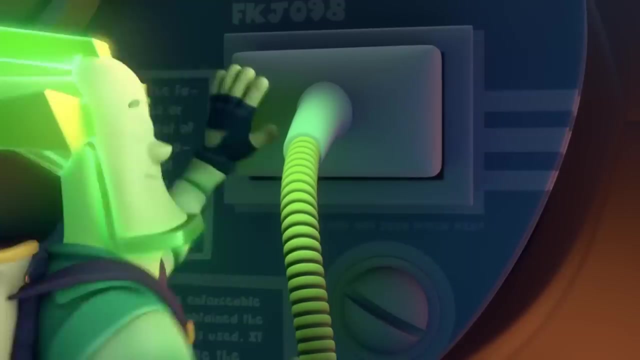 Of every single day. When there is an emergency, You know we're on our way. One, two, three Inside. we'll be All day and night. We fix things right. One, two, three inside, we'll be. 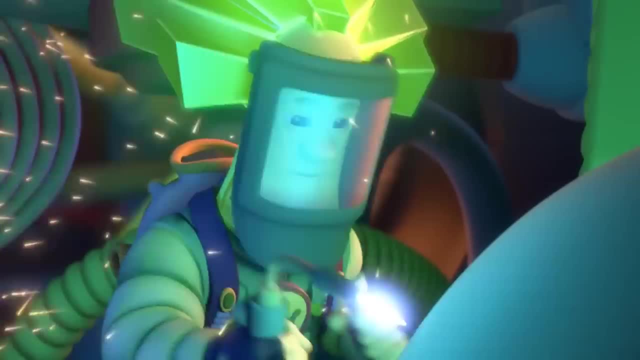 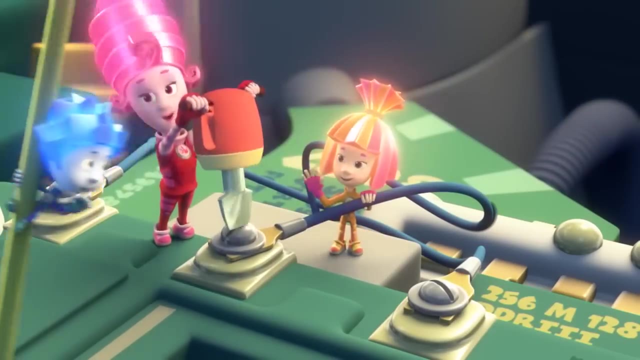 All day and night. we fix things right. We live to keep on working, And work for us is fun. So we'll just keep on working, Cause our work's never done. And deep inside of gadgets, If you look when it's dark. 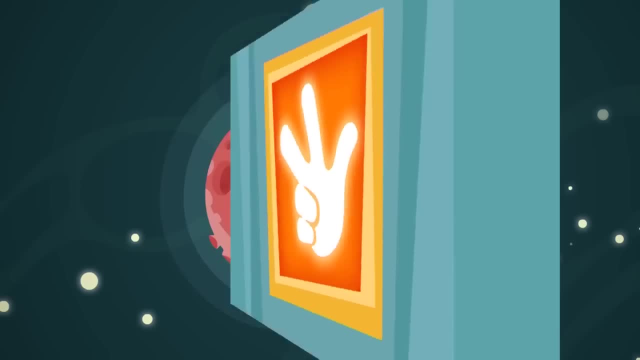 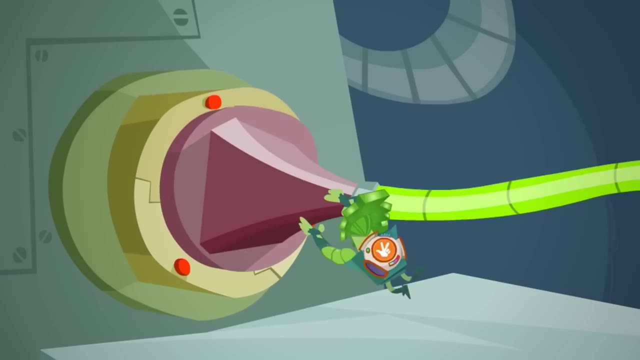 You might just see us face around Like multicolored sparks: One, two, three tideesh. Inside we'll be Tideesh To fix what's wrong. Tideesh Till it runs strong: One, two, three tideesh. 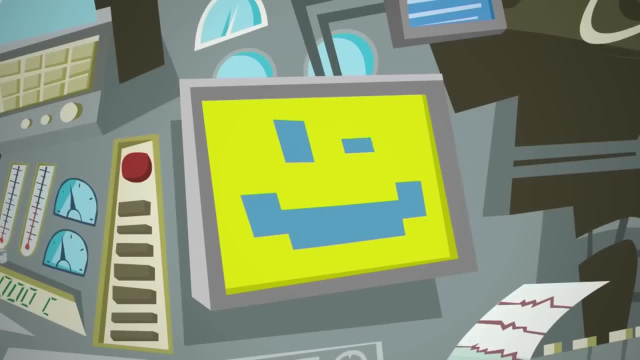 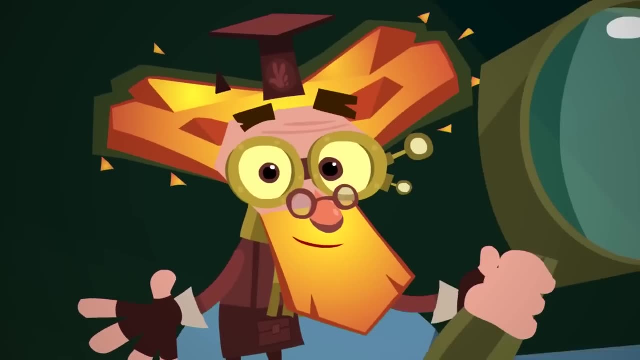 Inside we'll be Tideesh All day and night. tideesh, We fix things right: One, two, three tideesh. Inside, we'll be Tideesh To fix what's wrong. Tideesh Till it runs strong. 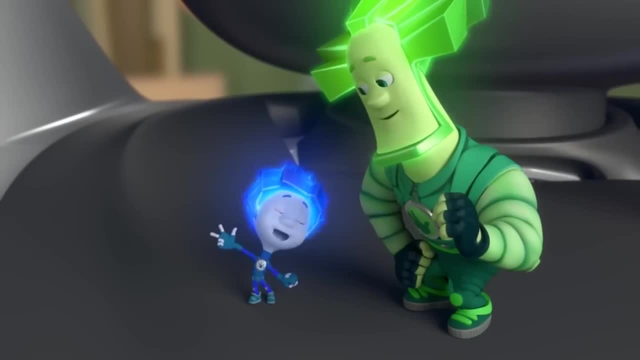 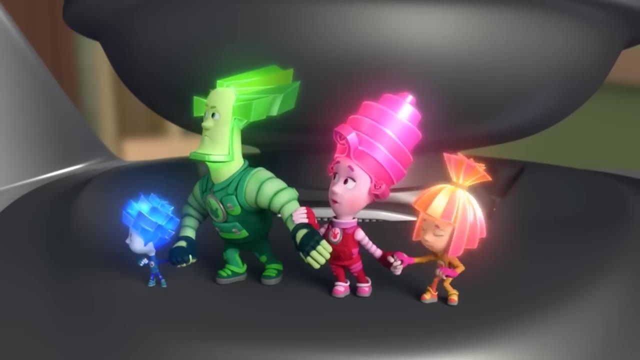 One, two, three tideesh Inside, we'll be Tideesh All day and night tideesh. We fix things right. Wow, you got it. We need to hide A robotazoid R300, I can't believe it. 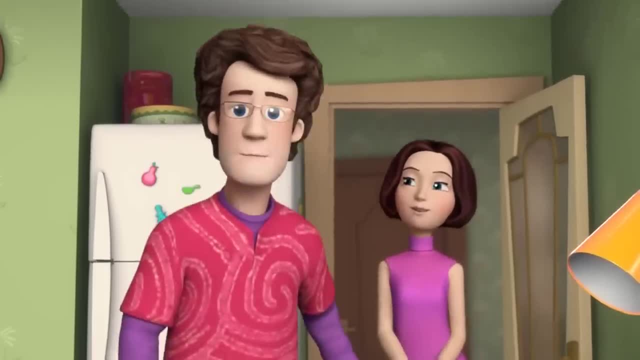 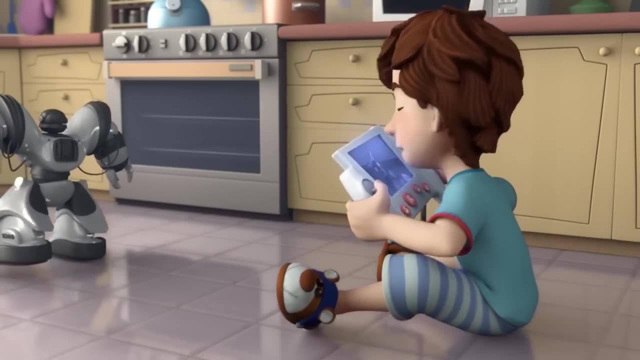 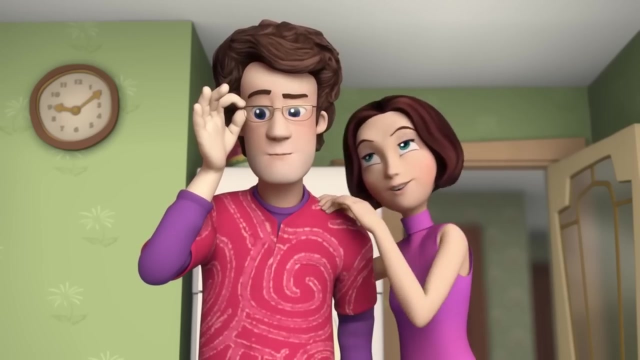 Well, happy birthday to you, Tom Thomas. I'm sorry, Tom Thomas. Last night your robot, you know I broke it, Dad, it works perfectly, Don't you see? I'm so proud of you. You fixed it. 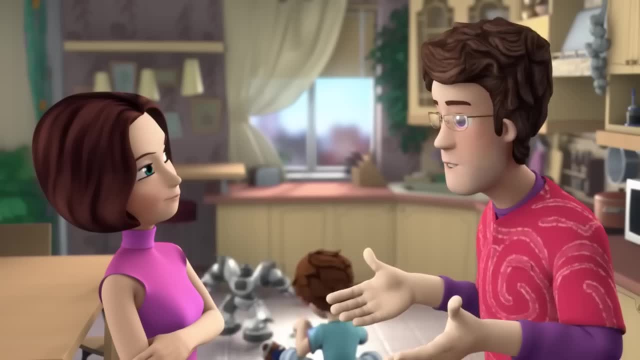 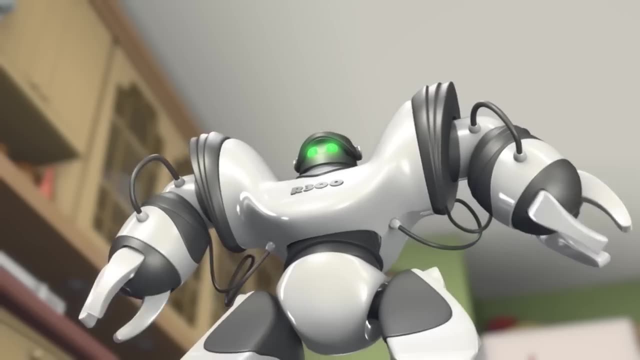 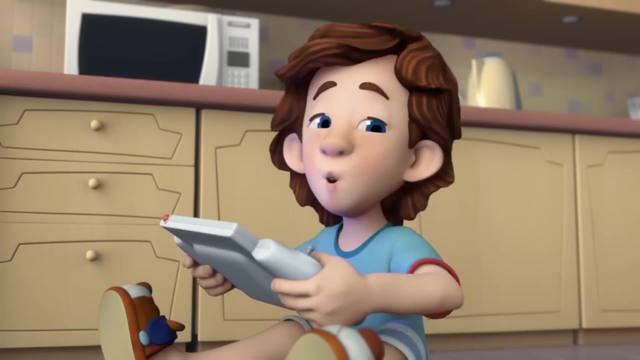 Shh, I couldn't fix it at all. I tried everything. Oh, you want to tell me that the robot fixed itself. What a joker. Woo-hoo-hoo-hoo, Mom Dad, thanks so much. I love it. 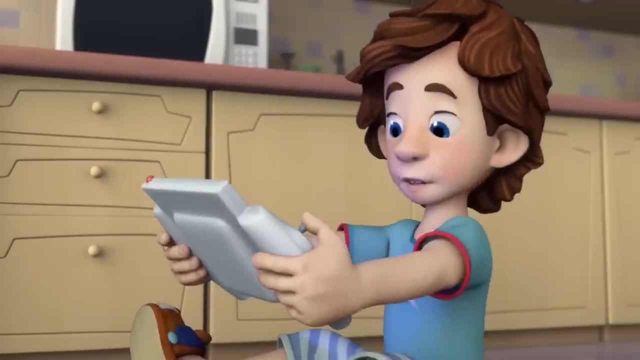 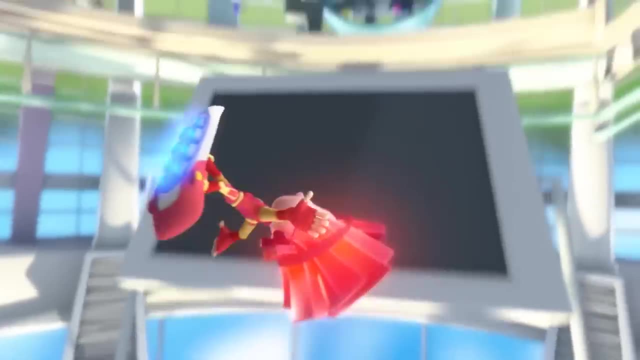 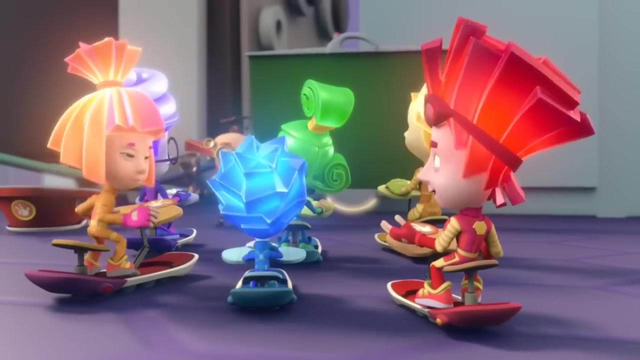 And how about thanking us? Thanks, I should have known it was you who fixed the robot. Happy birthday. Happy birthday, Quiet down. Get ready for your lesson. Be quiet, Quiet down please. Oh, it's so hot here. 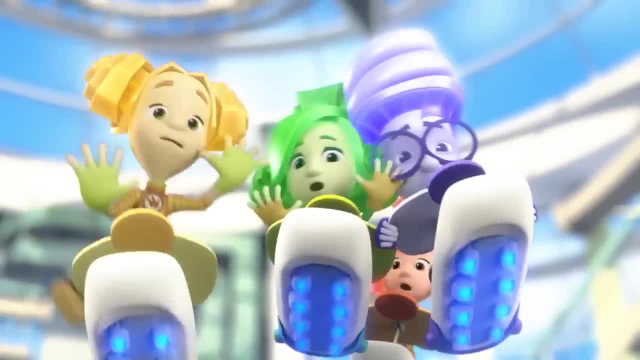 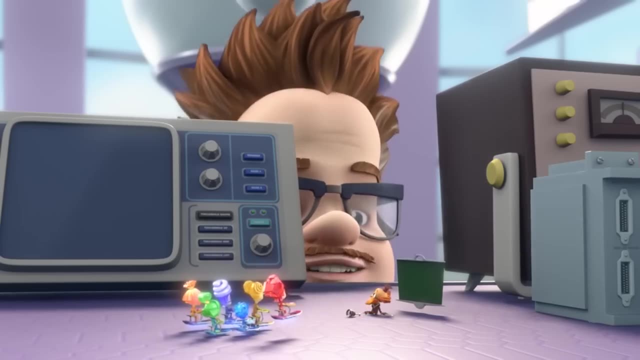 In today's class we'll learn about: Whoa, What was that? huh, It must have been an earthquake. Yeah, it was an earthquake. Hooray, Eh, sorry there, Professor. Ooh, I have to find an outlet so I can plug in this fan. 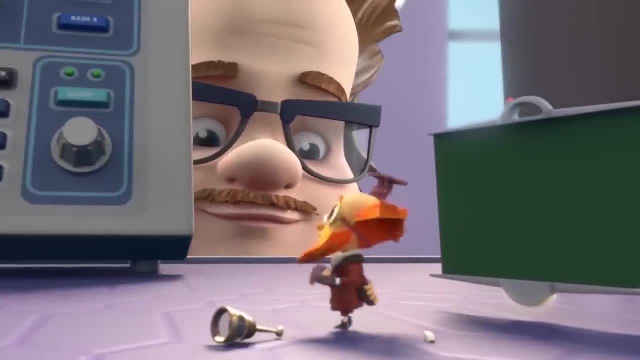 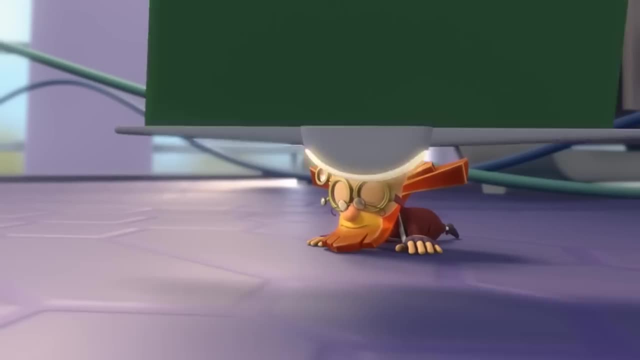 Ooh, it feels terribly hot. It sure does. Well, keep looking, You'll find one. Ahem, Now then where was I, Oh right, Today? Oh No, it's impossible. In this whole laboratory there isn't one free outlet. 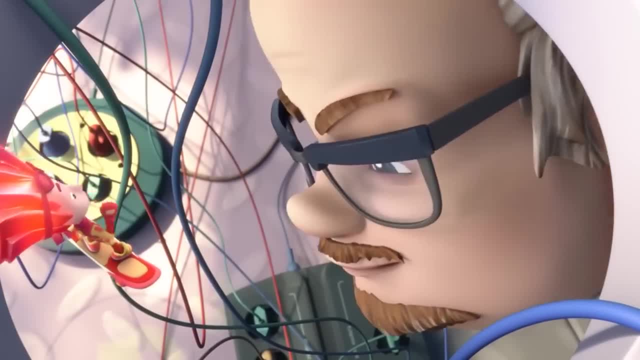 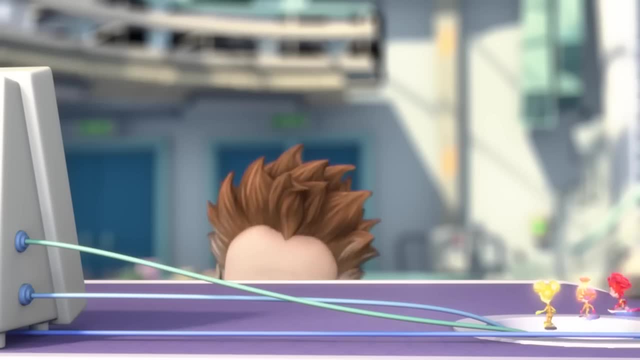 Look at this: Just pull out one of these wires and then you'll have a free outlet. I can't. I fear I could pull out a plug for something else, Something important. Ah, Volt himself would get all tangled up in these wires. 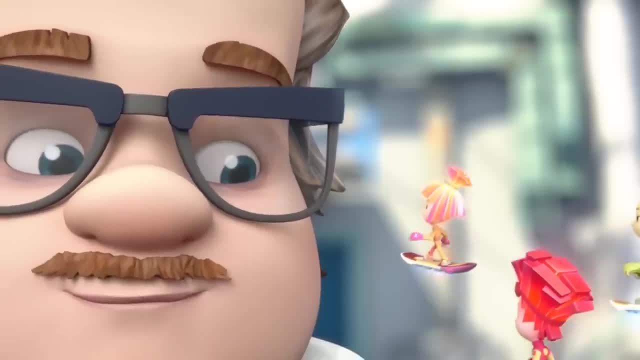 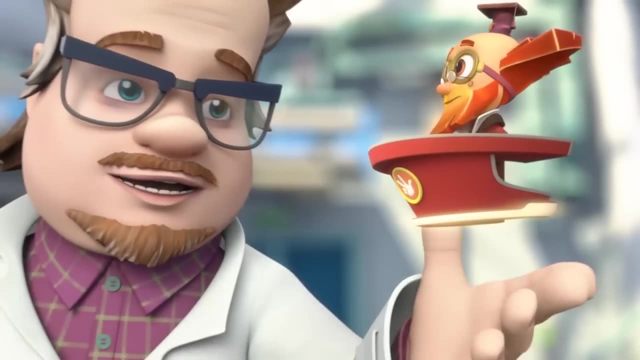 Don't worry about it, Professor Eugenius, We'll find a free outlet for you. That's right, my colleague. A cup of tea will do you good, so just go relax. Thank you, my colleague, And as always, I'm eternally grateful. 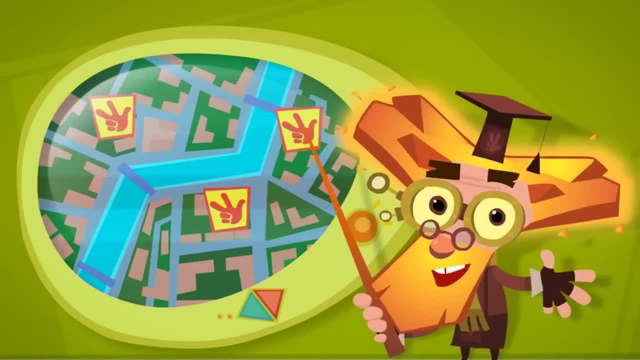 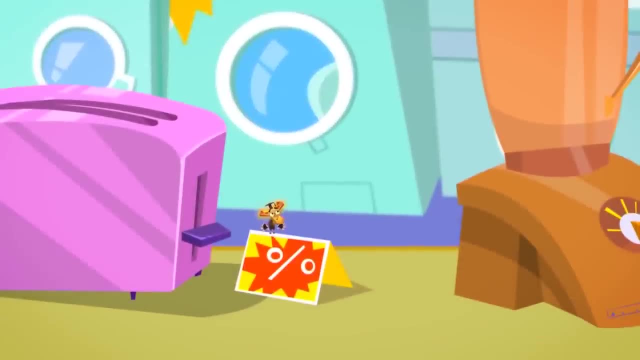 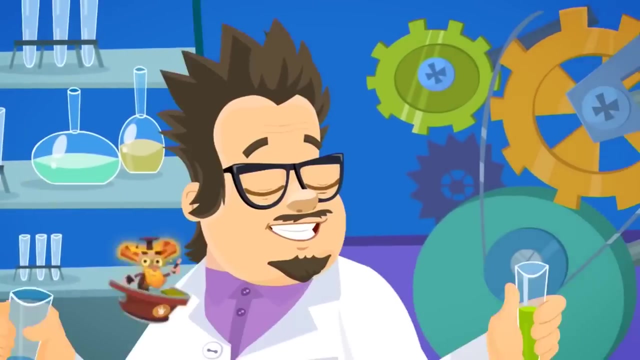 Fixies have opened schools for their children in all sorts of different places, like factories, stores and warehouses- Anywhere where there's lots of machines and appliances and places to hide from humans. And this is where we hold our school, right here inside the laboratory of Professor Eugenius. 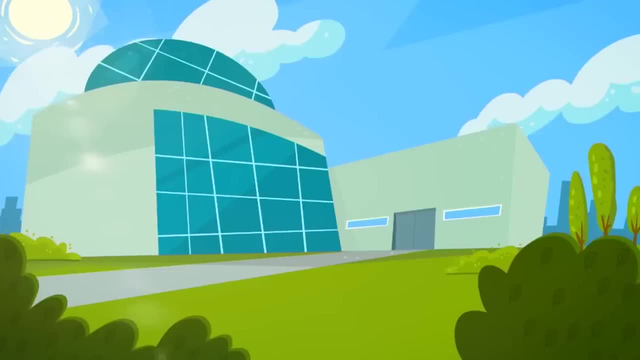 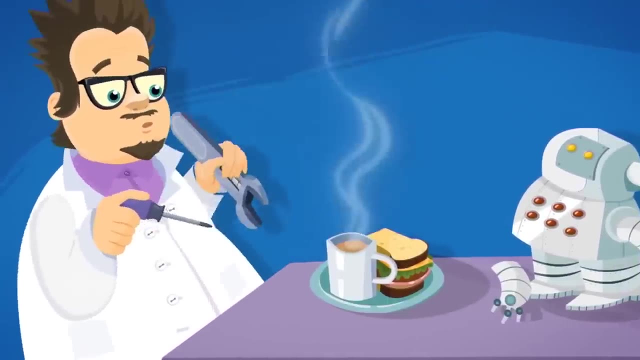 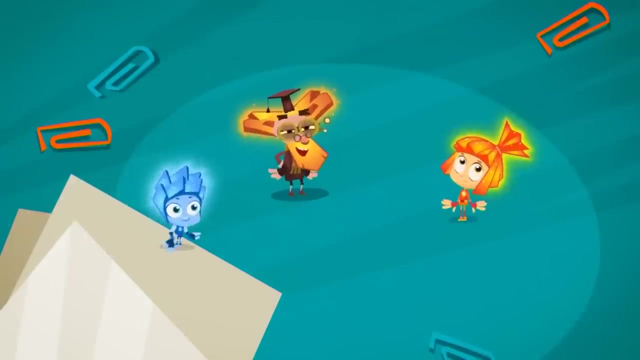 It's a fantastic place for me to hold class. Every day, new devices, materials, toys and even food are brought here for examination, And there are lots of scientific devices and tools to study here as well. But most importantly, we never need to hide from the head of the laboratory. 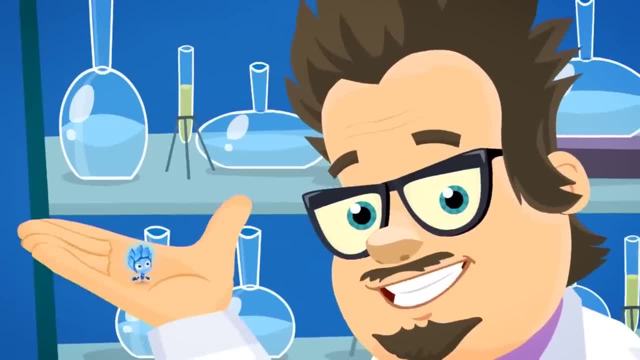 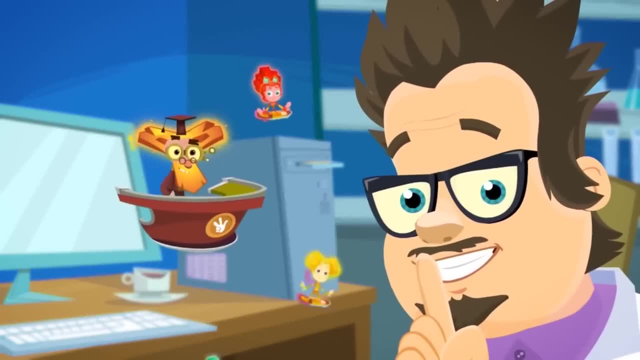 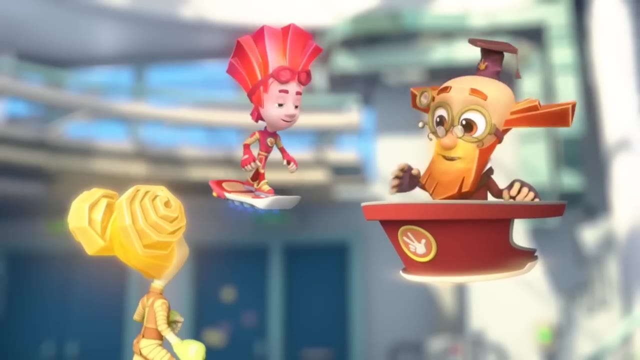 Because my colleague, Professor Eugenius, is someone I'm proud to call a friend. He loves Fixies, helps us any time we need and will never let our secret out. What should we do first? We have to start out with pulling apart these wires. 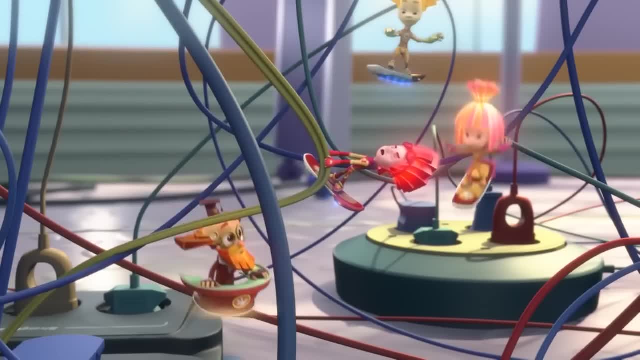 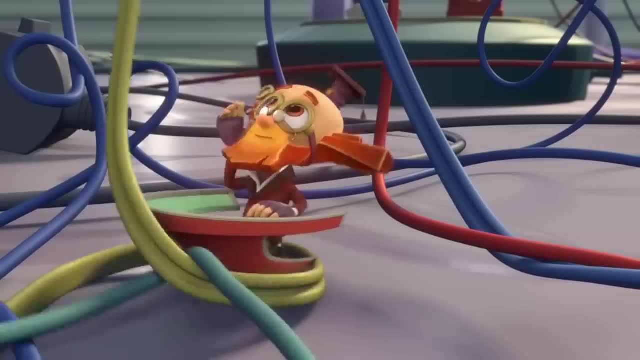 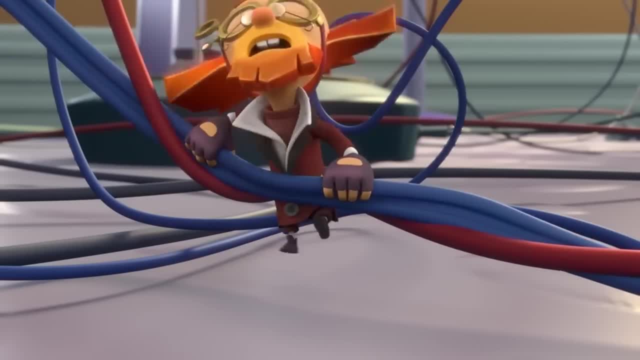 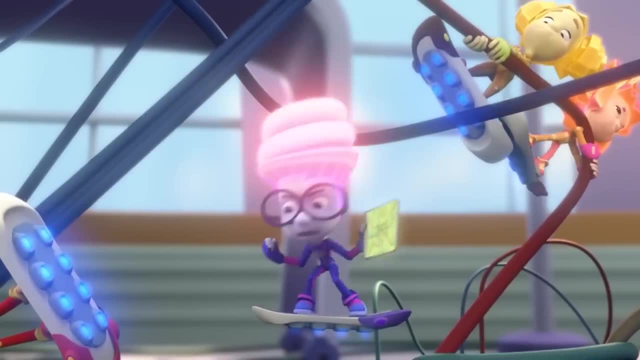 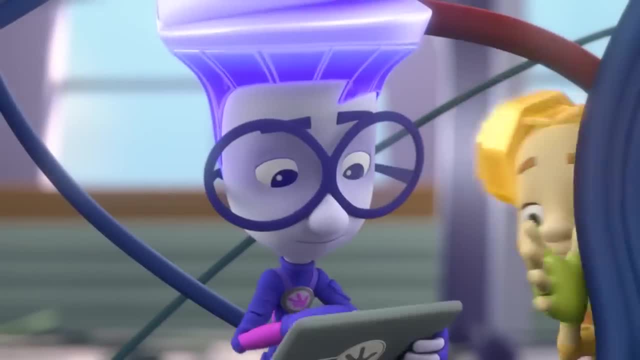 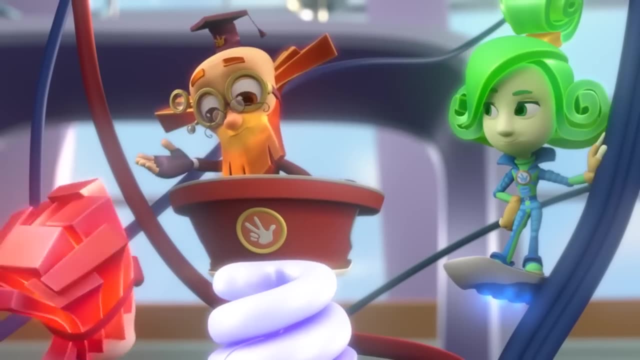 Thank you, digit Tideesh. Well, the way I see it, in order to get the knot out that's over here, we need to expand the loop that's over there And then push that wire through it And then do it again from the other end. 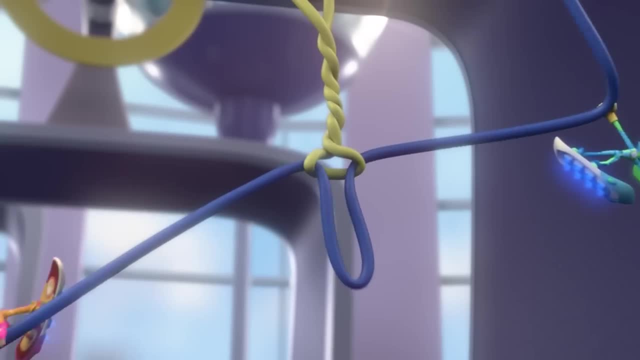 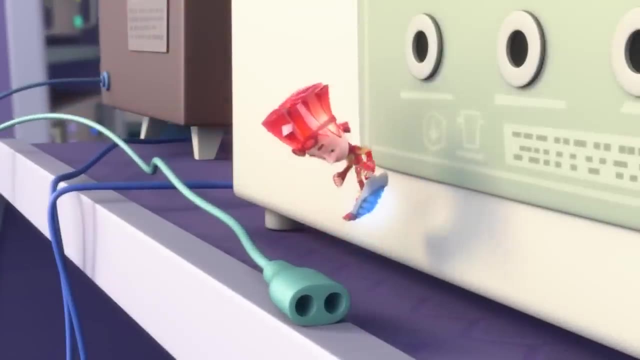 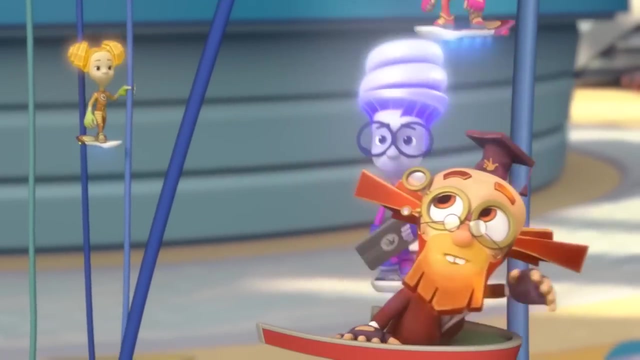 That's it. Very good, girls, Now pull it hard. Perfect, Hey, check it out. This green wire up here isn't plugged into anything, Then no one's using it, So that means we should go and pull it out from the outlet. 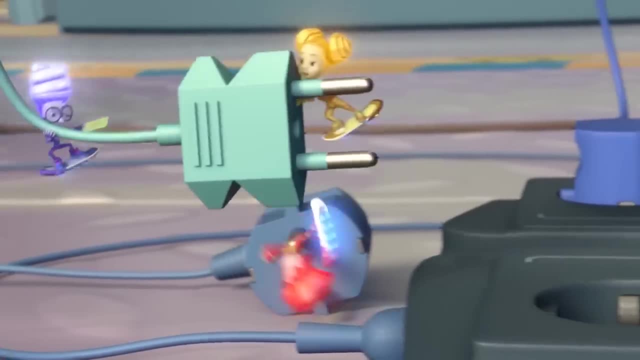 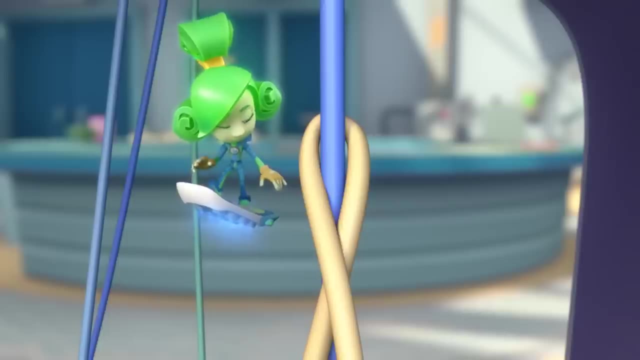 Got it. Oop Tideesh. Here's another wire that isn't plugged in. There it is. Here's another wire that isn't plugged in. I found another wire no one's using. Oh, I mean Simka, and I found it together. 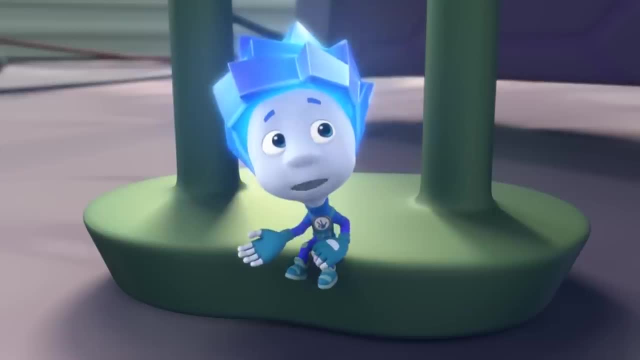 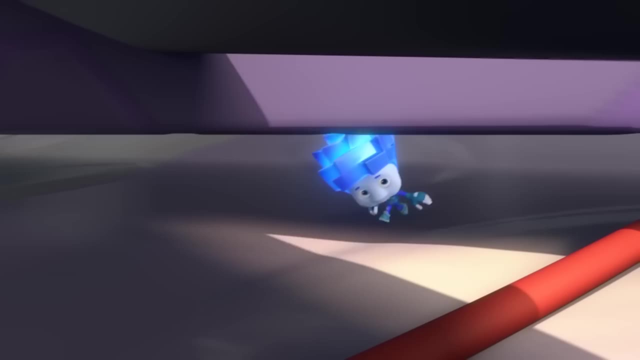 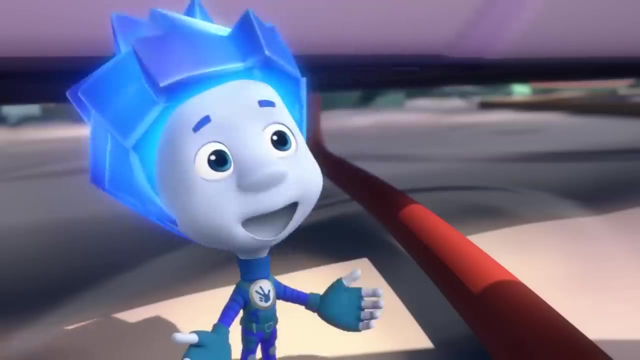 Nolik, why are you so upset? Because you guys are doing all the work. How about this wire? Nobody's checked it yet, Really, Oh wow, What Did you find? some treasure, Nolik. Uh-huh. There are six free outlets under here. 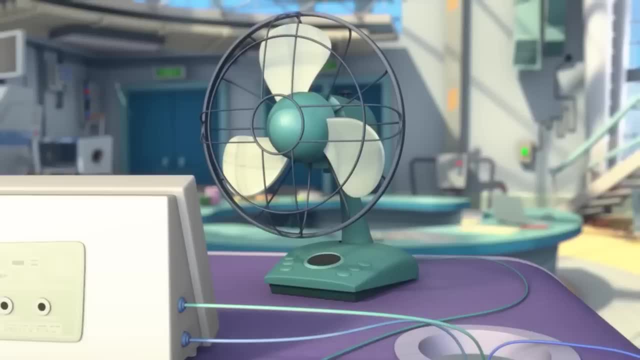 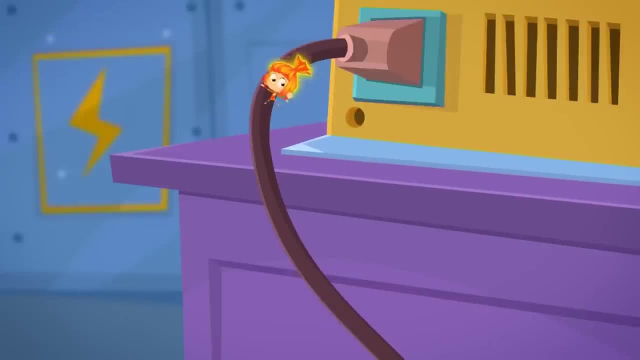 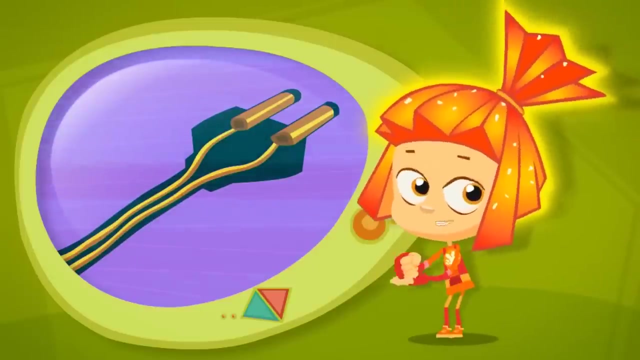 Great. Now Professor Eugenius can plug in his fan and his kettle and even his soldering iron. To get electricity to a device that doesn't use batteries, you need to plug a pair of wires into an outlet, But it's important not to let the wires touch one another. 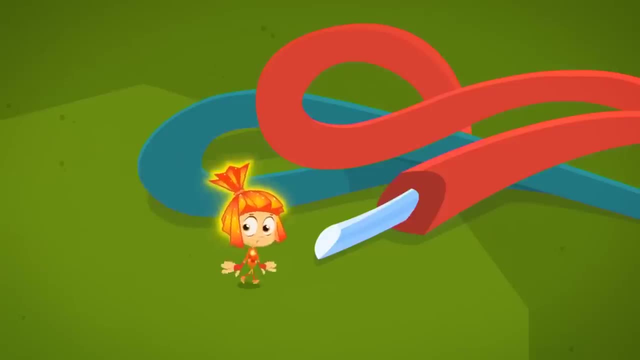 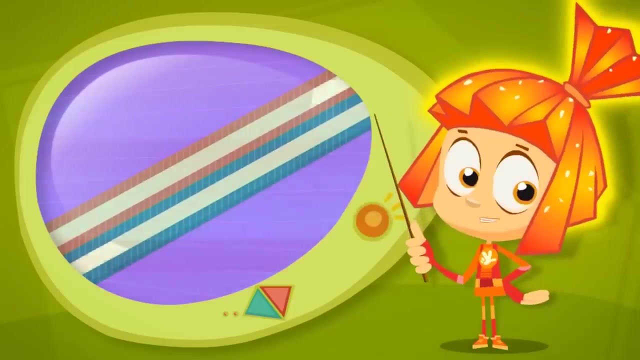 or the electricity can burn them out. That's why wires are covered in plastic or rubber, so the electricity won't pass from one wire to the other Or to us when we touch them. So always be very careful with wires And never, ever touch a bare wire. 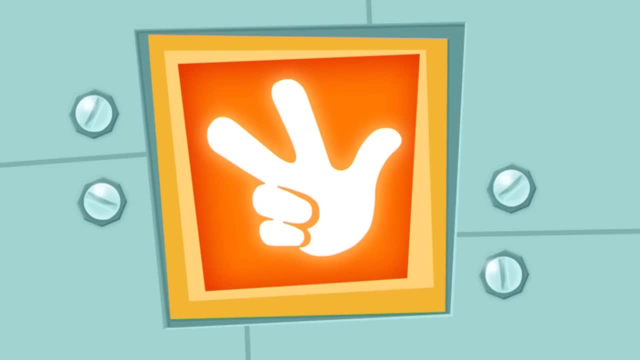 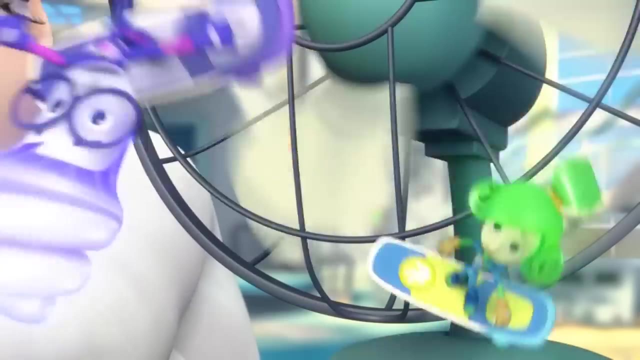 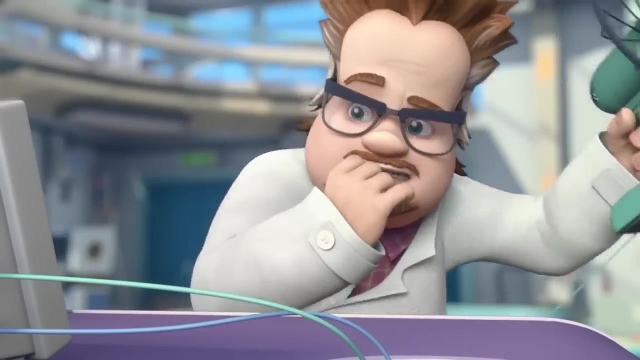 You could get killed by the electric shock. Oh, what would I do without my wonderful friends? Thank you, Ah sorry, I just I didn't. I wanted to. I should go Go ahead. that's a great idea. 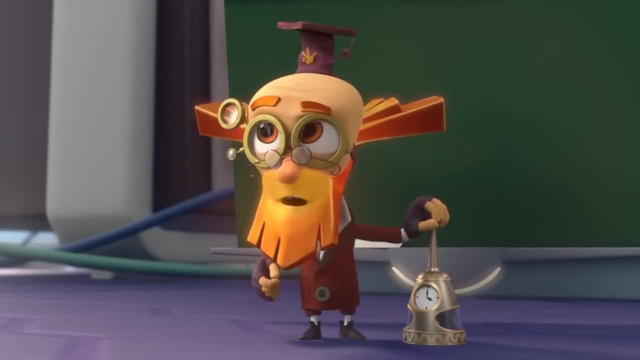 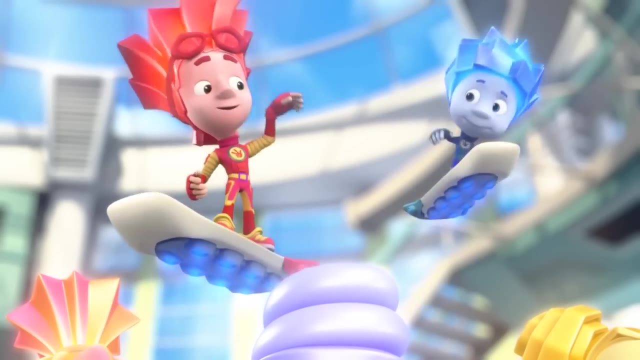 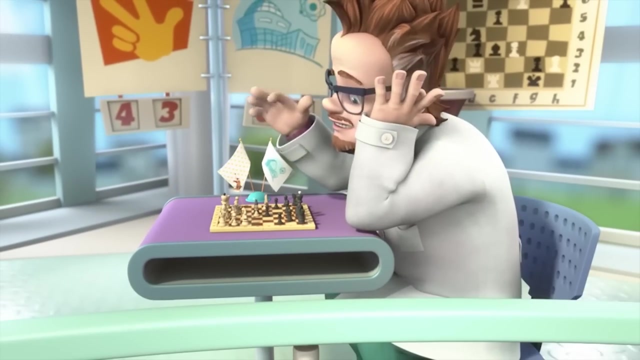 And we'll start our class. Eh, what were we talking about? All about wires? Well, it looks like our class is over Time to go play. How about that? Then I'll play my pawn And I'll play my pawn. 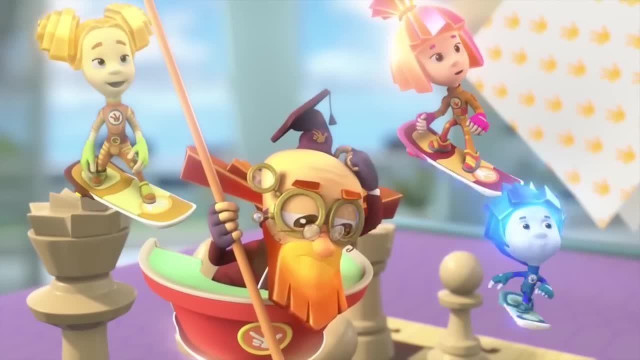 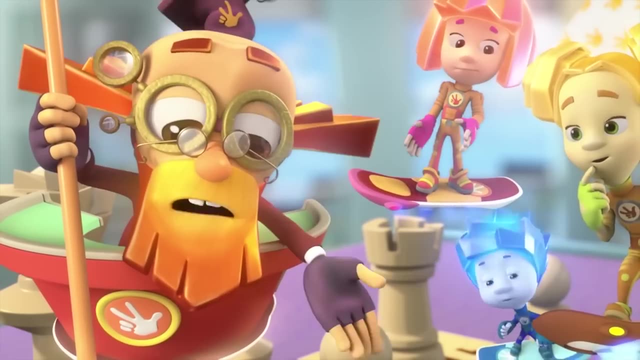 Grandpus, we need our spool and it's missing. Congratulations, Professor. have you seen it anywhere, The spool? I haven't seen it. We're playing chess, can't you see? Do you like board games, Like dominoes, for instance? 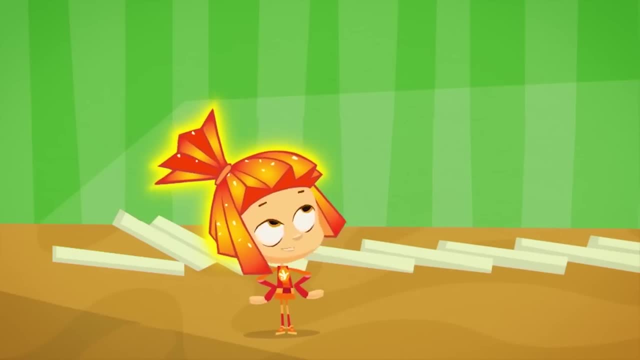 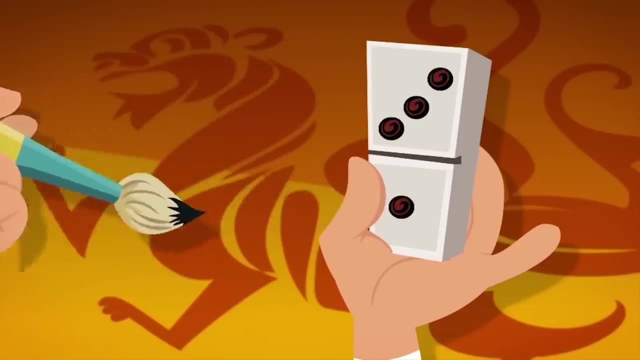 Just about everybody has played it, But do you know where it came from? Dominoes was invented by the ancient Chinese. They made tiles and decorated them with dots, like on a pair of dice, And this is a game that looks a lot like checkers. 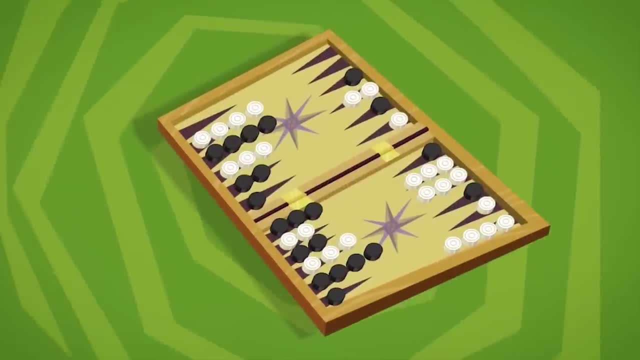 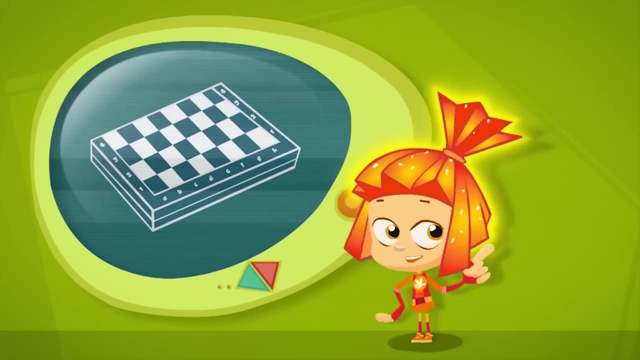 but it's a lot more challenging. It's called backgammon. Backgammon originated in Persia and from there it spread all over the world. But the most challenging game of them all is the game of chess. Chess was invented in India. 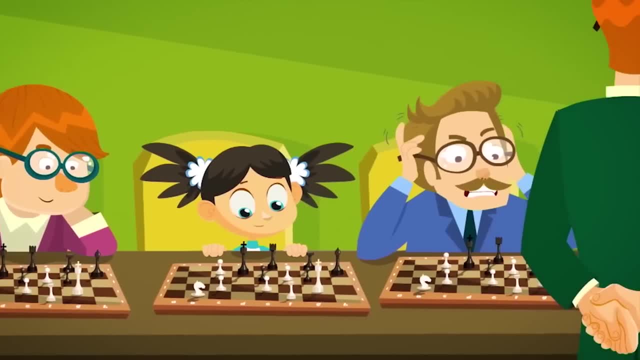 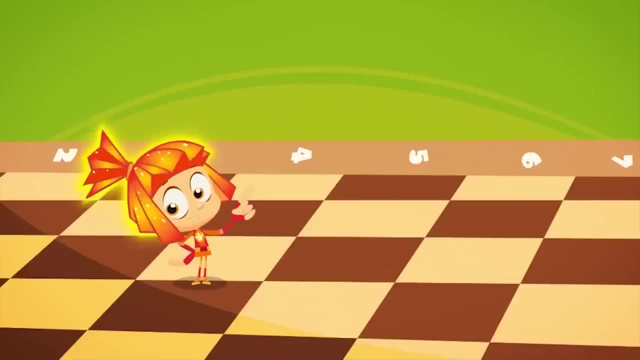 and today the game of chess is loved in every country. It's played by adults, by children and even by computers. Chess is a real sport. But the most important thing for playing chess is not the power in your arms, but the power in your brain. 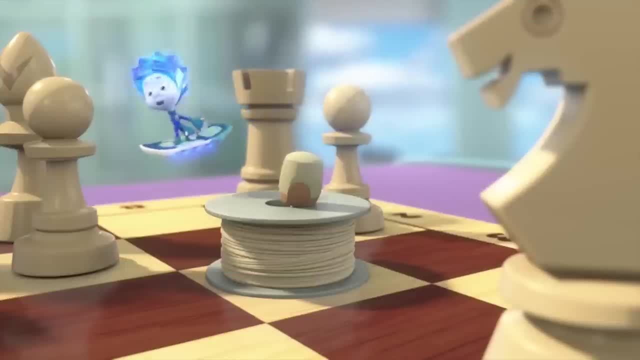 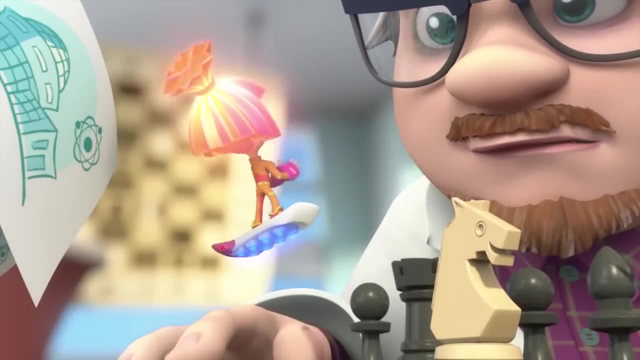 To use it. you need to use it And this is how you can use it. you can use it all day, when you never thought of it before. Hey, look, I found it. Hey, what's going on? That's our spool. 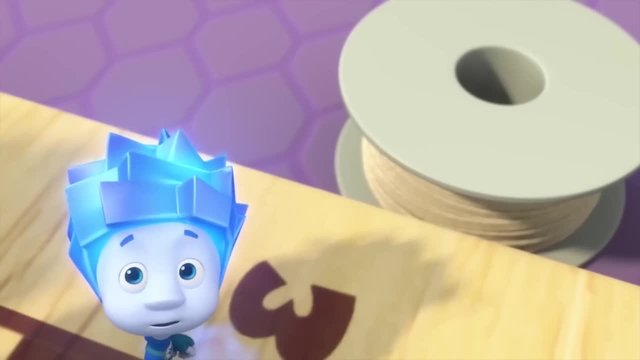 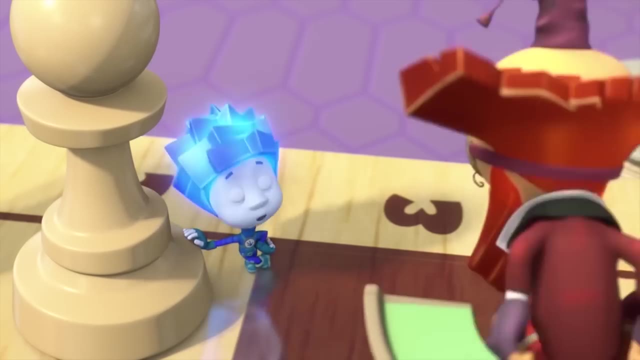 Please let us take it back. There's something we have to do with it, But we're using it, Can't you wait? It's a replacement for the missing pawn. Nolik can work for a while as the pawn's replacement. 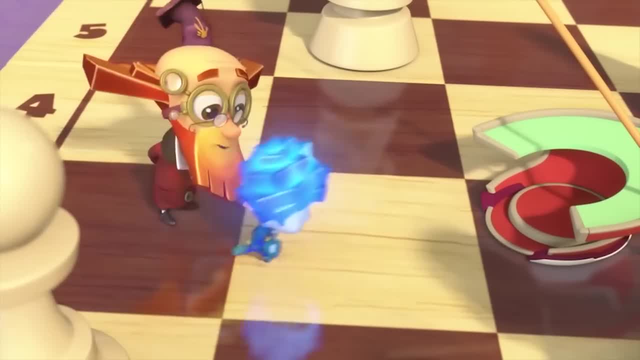 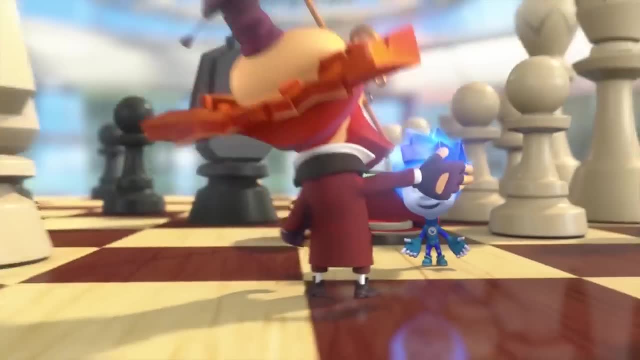 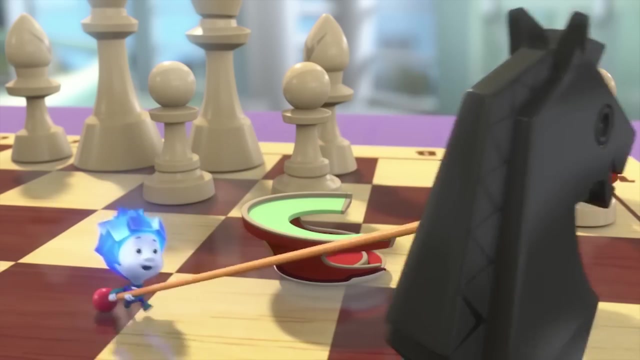 Yeah, And you stand right over here. One, two, three, up we go Class. So how do we play? You're going to play for the whites And now I'm going to capture your knight And we we're going to knock over yours. Take that. 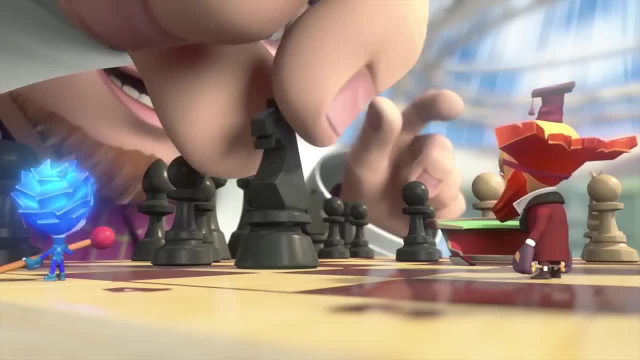 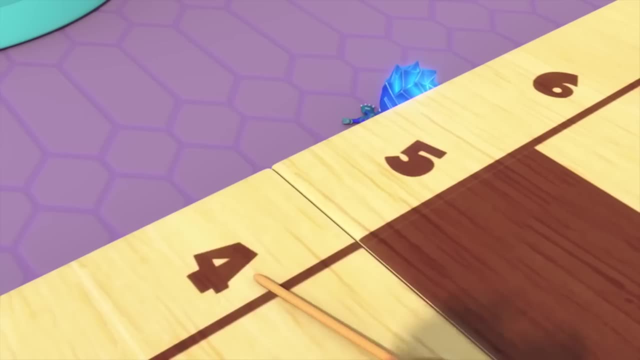 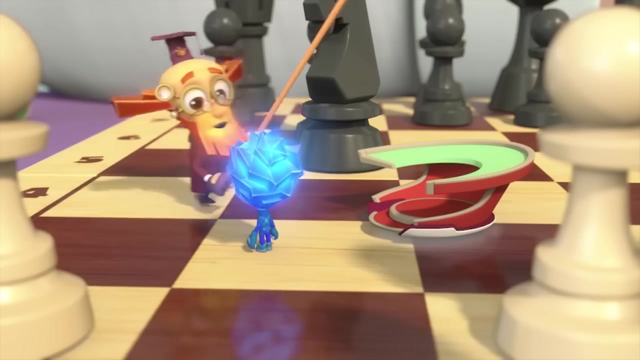 Whoa, whoa, whoa young man, Slow down, It goes back here. Ugh, Nolik, get back to your square. What for Pawns don't move like that? Then how do they move? Only one square per move and only forward. 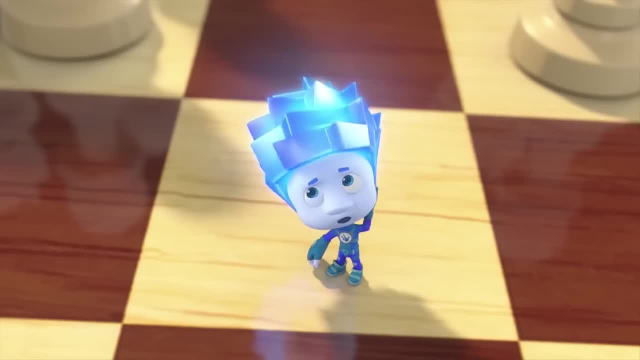 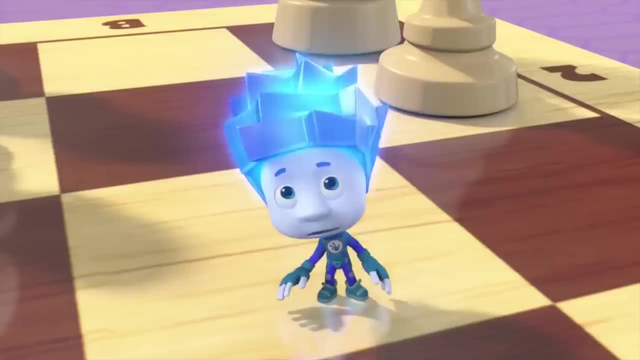 Of all of the pieces, the little pawn is the weakest. What a mess. So which one's strongest? huh, This, It's the queen. She's the most dangerous threat to the other king. Aw, how come I couldn't be queen? 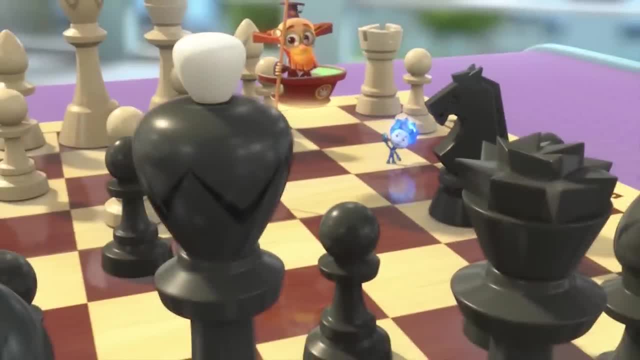 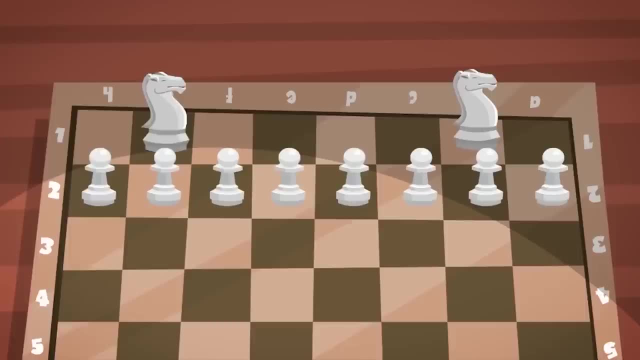 Then that black king, That black king would have to deal with me. Oh yes, In chess each player has a black or white army with eight pawns, two knights, two bishops, two castles and a queen. All of them work together for their king. 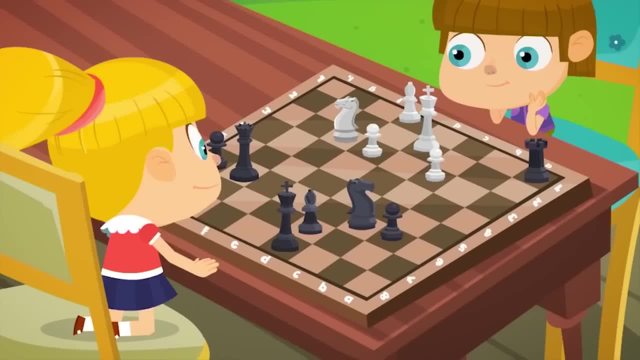 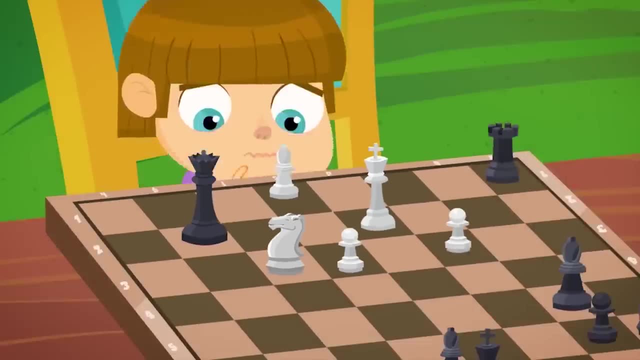 trying to protect him while attacking the enemy's king. If the king finds himself in a position where he can be captured, the attacking player says check, And if the king finds himself with nowhere to run from the attack, it's called checkmate. 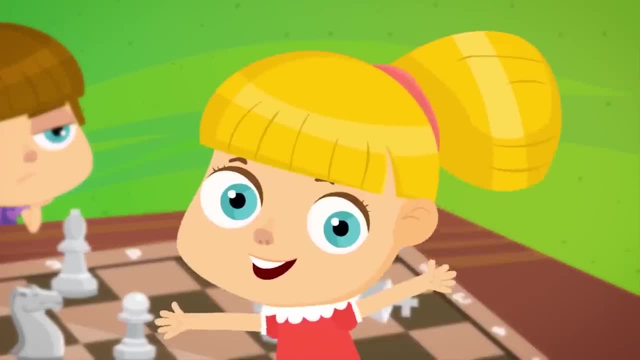 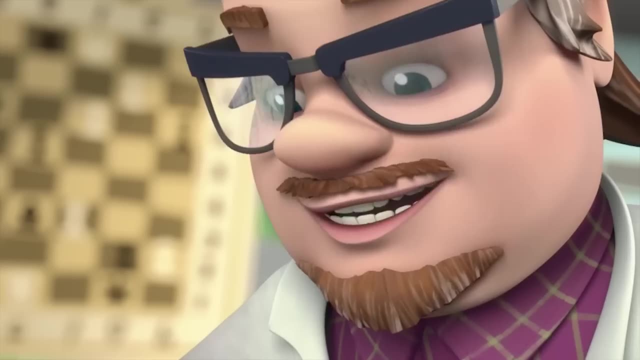 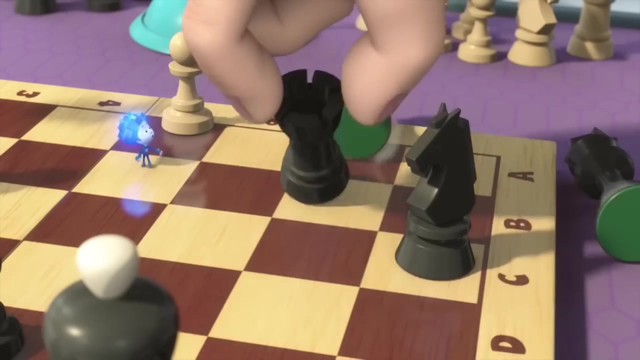 Whoever checkmates the other player's king first is the winner. I'll move my queen And me my queen. Then I'll just capture your queen Really, Then I'll just capture yours, Grappus, should I go now? 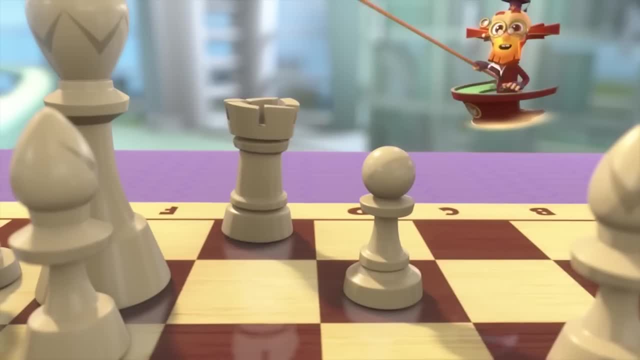 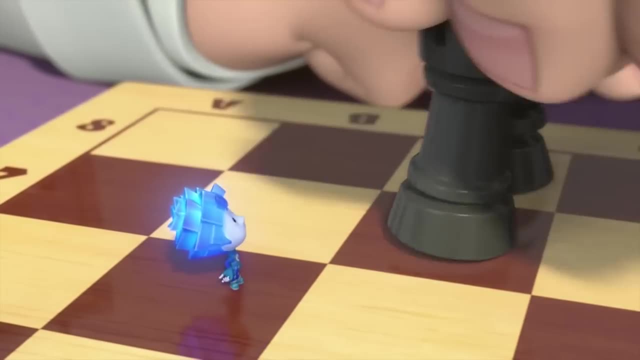 Not yet. So do you feel like surrendering? You're kidding, do you? Nolik forward, Hooray, We'll step aside Forward, Aha. Next I'll go and capture the knight. He got away. 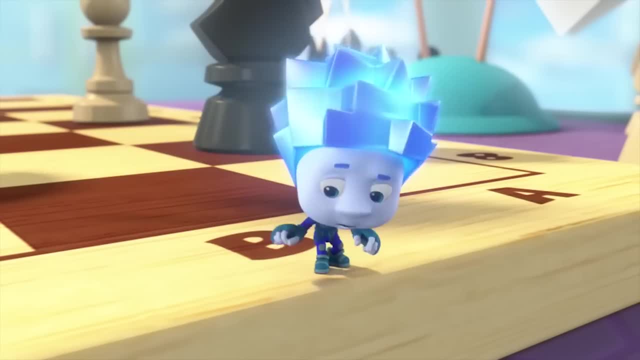 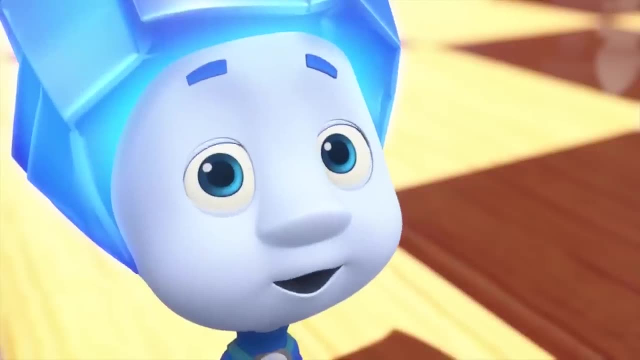 All right, pawn and once more, go forward. Grappus, where do I go now? Don't you see the edge? Don't go anywhere Now. you're the queen. What? The rules of chess say that if a pawn makes it all the way to the other side. 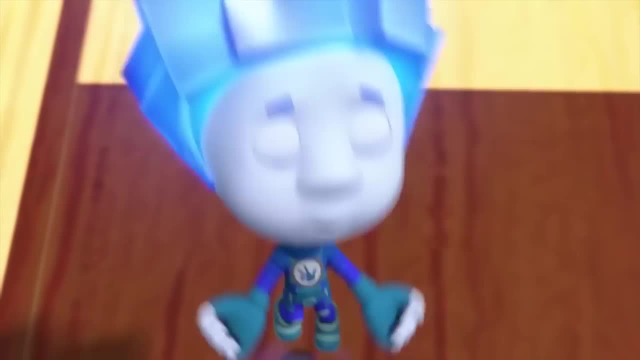 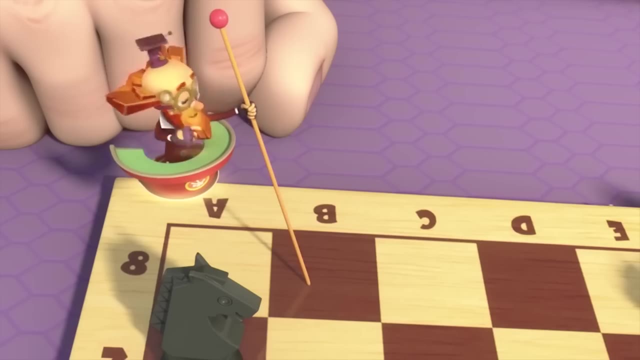 he can become anything that was captured earlier. Hooray, Then I'll be the queen And I'll be the strongest piece in the whole game. Hey, queen, get back here In case you don't know. this isn't over yet.